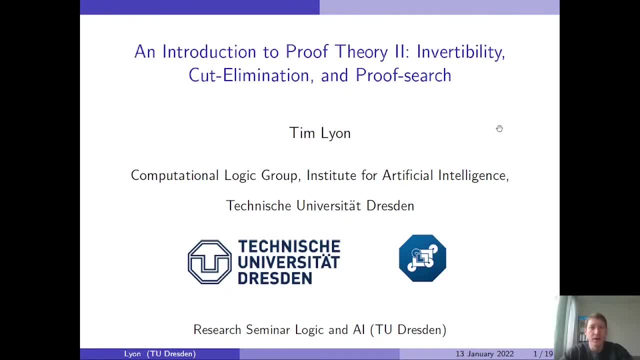 Today I'll be giving part two of an introduction to proof theory. This will be a continuation of the first part of the talk, an introduction to proof theory, one on the sequent calculus, and we'll build off of what I discussed there. Today I'll be discussing three different concepts, namely invertibility, cut elimination and proof search, specifically with respect to the sequent calculus that was introduced in the first talk. 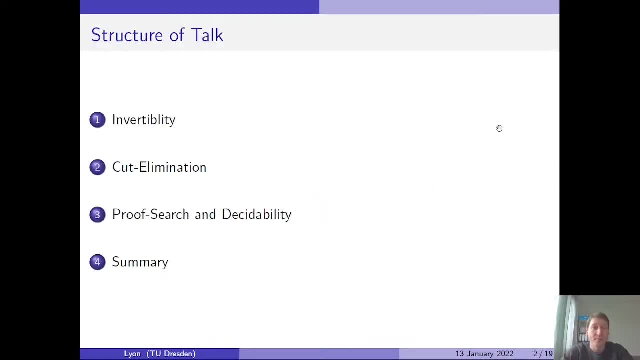 And I'll also be mentioning results, which we'll discuss there as well. Now, just to give a small overview of the talk, what I'm going to do first is discuss what are called invertible rules. Invertible rules are rules in a sequent system where the derivability of the conclusion implies derivability of the premises. 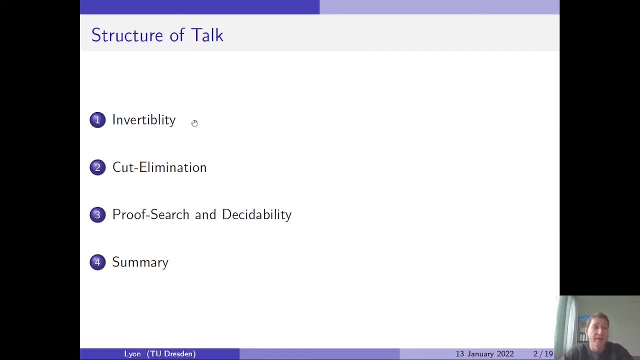 And these are useful for various reasons which I will be going over in that first section. This also will be used to help establish what is called cut elimination. So, although I'm not going to prove that the cut rule is eliminable in our system in general, 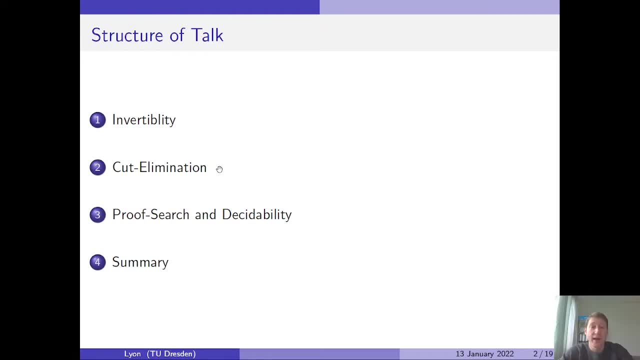 what I will be doing is I'm going to be discussing the rules of the sequent system, And that is looking at various cases and showing how cut can be removed and give a general idea about how cut elimination works. After that, I will then talk about how aftercut has been eliminated from our system. 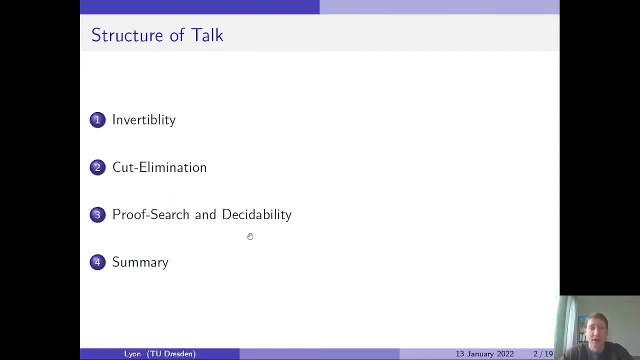 Our system is what is called an analytic proof system, which oftentimes means that it has the sub-formula properties. This is what we will mean by analyticity here, in the context of this talk. I'll then explain how, just by observing the structure of the inference rules of the system that we can conclude that 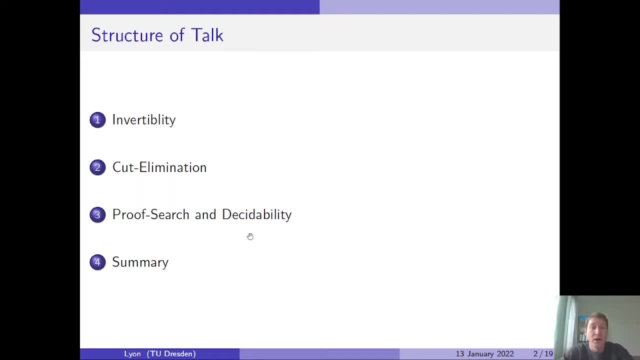 classical propositional logic is decidable, something which we already know and which is well known, but something which sheds light on how this proof theoretic method can be used to establish decidability of logics. After that, I will then explain and give an example of proof search showing how this works. 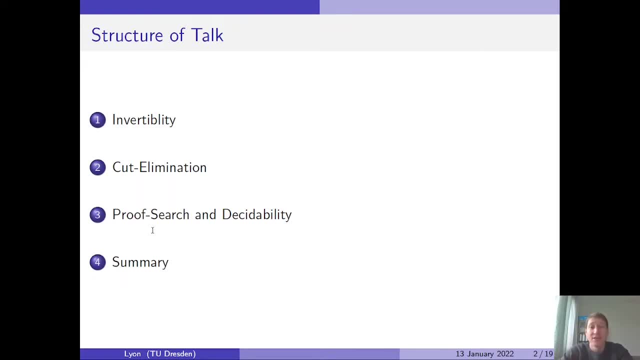 In other words, this will be, or is, a type of a decision procedure or decision algorithm which decides a logic. So I'll give an example of proof search showing how the decision procedure can be rewritten for classical propositional logic, and this can be adapted to other settings as well. 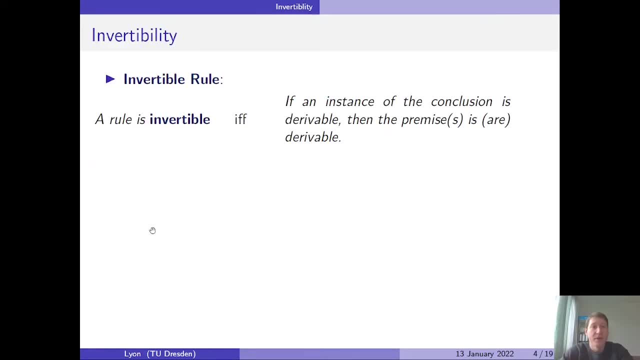 At the very end I will summarize everything. Okay, so what is an invertible rule? Here I will discuss two different notions of invertibility. The first notion is defined as follows: A rule is invertible if, and only if, an instance of the conclusion is derivable. 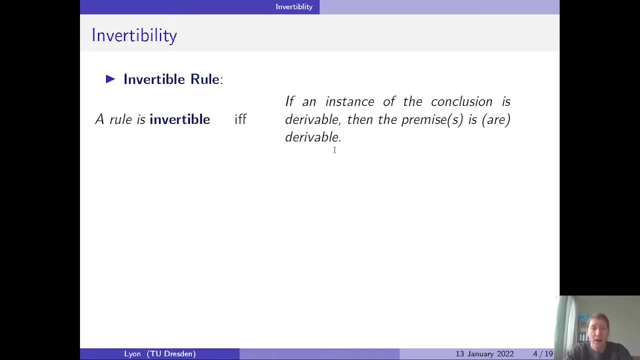 then the premises are derivable as well. In other words, one way to put this in short is that derivability of the conclusion implies derivability of the premises. There also is a stronger version of invertibility, referred to as height-preserving invertibility, or HP invertibility. 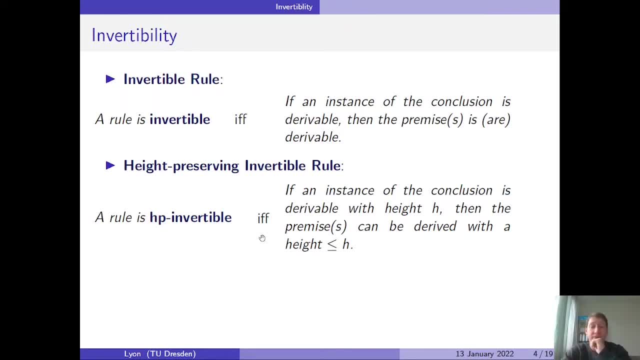 A rule is going to be HP invertible if, and only if. whenever an instance of the conclusion of the rule is derivable with a height h, then the premises can be derived with a height less than or equal to h. In other words, what this means is that derivability of the conclusion with a particular proof implies derivability of the premises. 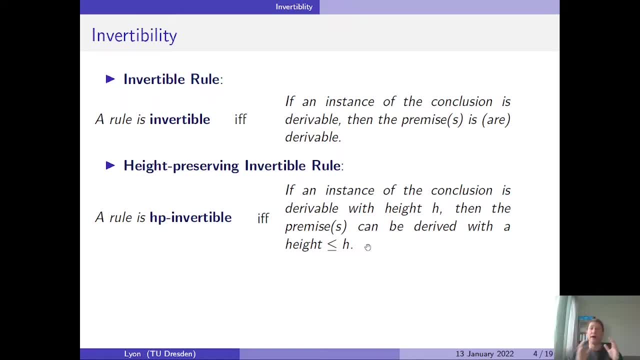 and the height of those derivations is bounded by the derivation height or the conclusion of the rule. Now, what are the benefits of invertibility and HP invertibility? Well, it turns out that invertibility can be quite useful in establishing HP admissibility. 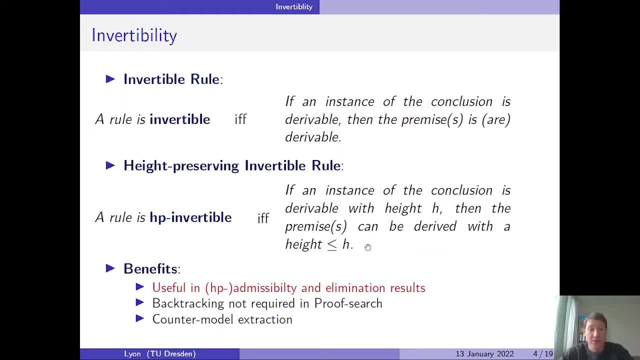 or just a bit more. In the first lecture I talked about the importance of invertibility in the proof system, So this deals with showing that certain rules in your proof system are redundant. This is discussed in the first lecture, So if you'd like to see how certain structural rules in the sequent calculus are admissible or eliminable, 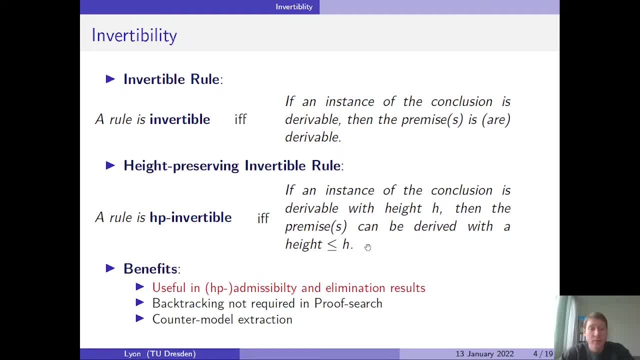 this is discussed there. Now, with respect to our sequent calculus, the weakening and contraction rules are HP admissible and eliminable in their own right. But if you deal with more complex proof systems, you have to show invertibility of rules before you can show, for example, contraction admissibility. 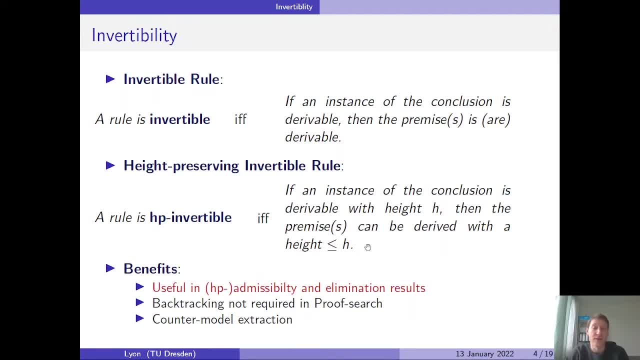 So this really is useful in helping establish these results And, as we'll see over the course of the next few slides, or momentarily showing elimination in our sequent calculus, depends on or uses the height-preserving invertibility of certain rules in our proof system. 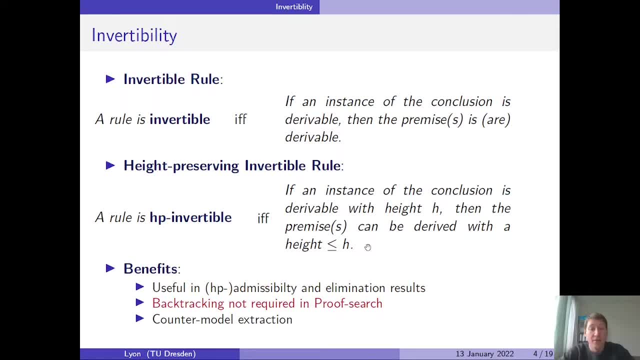 Another thing which is very nice is that if you have that, your rules are invertible, then this means that if you do proof search, meaning if you give me a formula or give me a sequent and I apply the rules in reverse, trying to construct a proof of that formula or sequent- 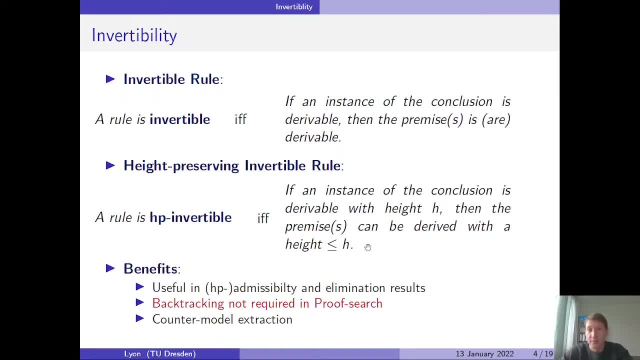 backtracking is not required in that process. So, for example, imagine that I'm trying to construct a proof or extract a proof from a given sequent or formula by applying inference rules in reverse. If at some stage of this process, I have a rule R1 that's applicable and a rule R2 that is applicable, 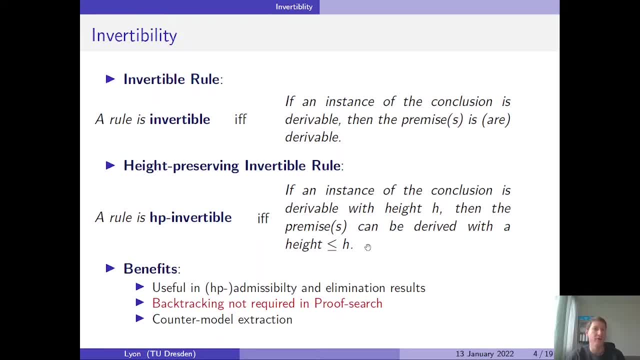 if these rules are not, or if one of these rules is not invertible, then that means it's not the case that the validity of the conclusion implies the validity of the premise. So if I apply this rule in reverse, I might go from a stage during proof search where I have a sequent which is valid or which is derivable. 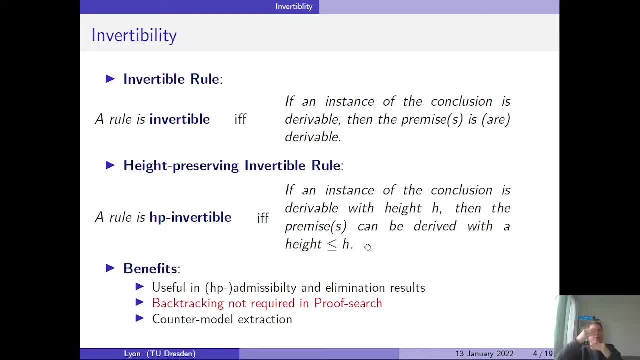 and then what I deduce by applying the rule in reverse, one of the premises is actually not derivable or is not valid, And so what would happen is, after I would complete my process of extracting a proof, it could turn out that that proof is not actually a proof of the conclusion. 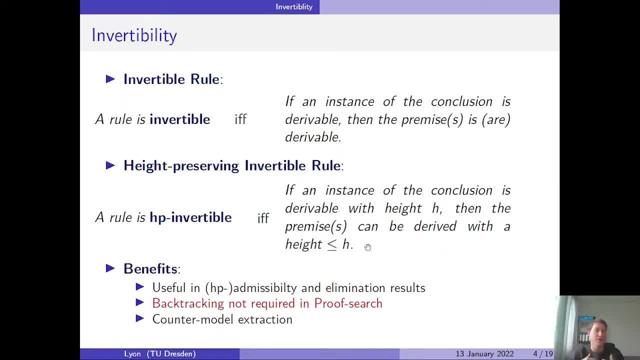 Now this doesn't necessarily mean that that sequent the conclusion of the proof is not provable. What it means is that when I had that choice of applying either the first rule or the second rule, I made the wrong choice, And so I then have to backtrack in my algorithm, go back to that step and apply the other rule instead. 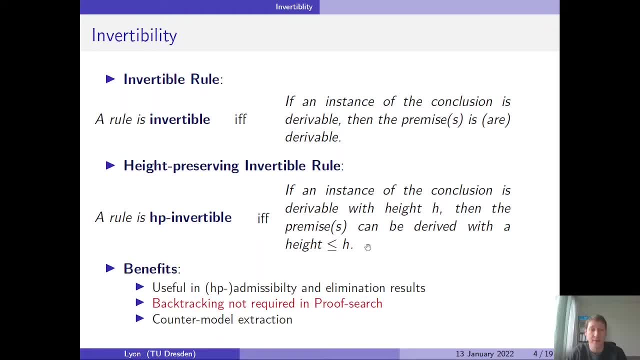 And this could, of course, make proofs valid. It could make proof search rather complicated. Now, to make proof search more intuitive for the audience, what I'm going to be doing later on is give an example of successful and unsuccessful proof search by making use of our sequent calculus LCP. 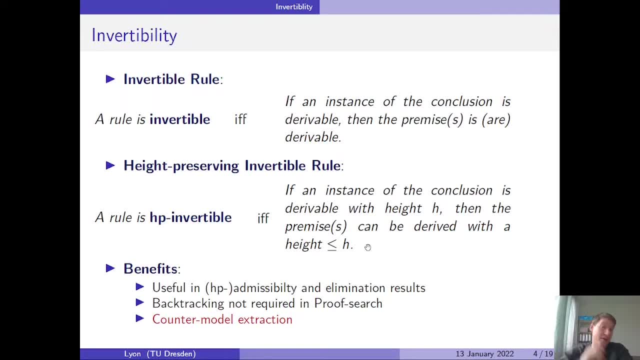 Now, another thing that's useful regarding invertibility is counter-model extraction. Now, if a rule is invertible, what it means is that the validity of the conclusion of a rule implies the validity of the premises. So if you think about the first rule, 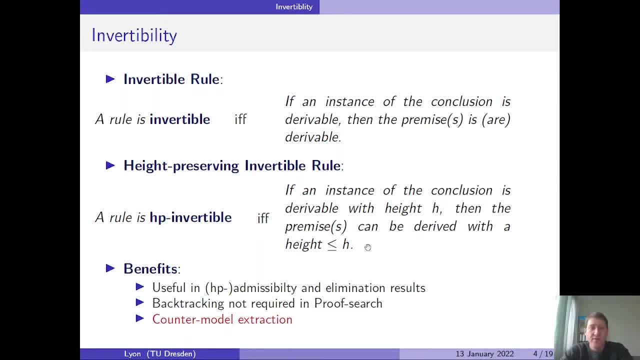 the contrapositive of this. what this means is that if one of the premises of the rule is invalid, then the conclusion is invalid. So if I do proof search and I obtain something which looks like a proof in my sequent system, 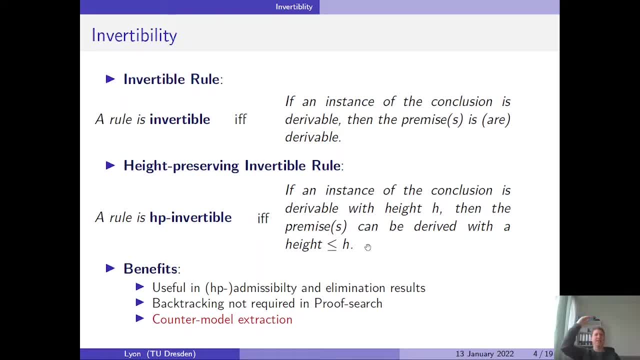 and one of the initial sequence is not an axiom, but is something which is invalid. I can construct a counter-model for it And since the invalidity of something is carried downward in the proof, the invalidity will be carried downward to the conclusion and the conclusion will be invalid as well. 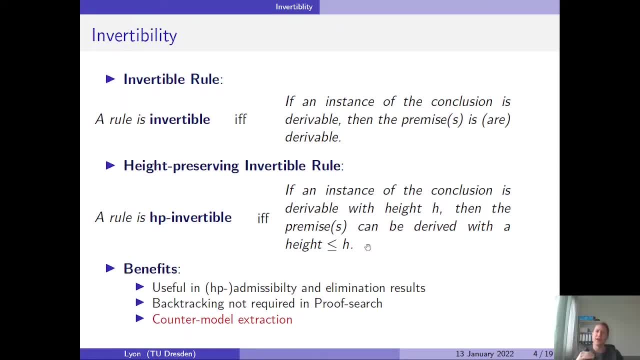 So if I have a counter-model, well, so long as the rules are of a nice shape, which they are in our case, be a counter-model of the conclusion as well. Again, I will give an example of this later on in this talk to get the idea across better. 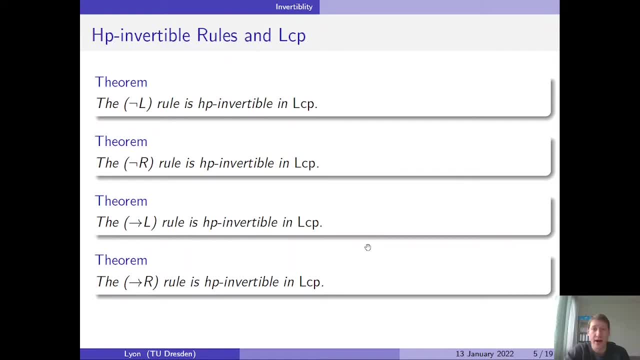 Now it turns out that in our sequent calculus all the logical rules are height-preserving invertible, both the negation rules and the implication rules. So what I'm going to do now is explain how we can prove that the negation left rule is height-preserving invertible. 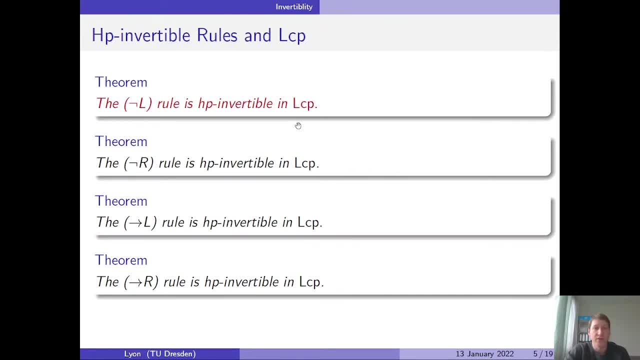 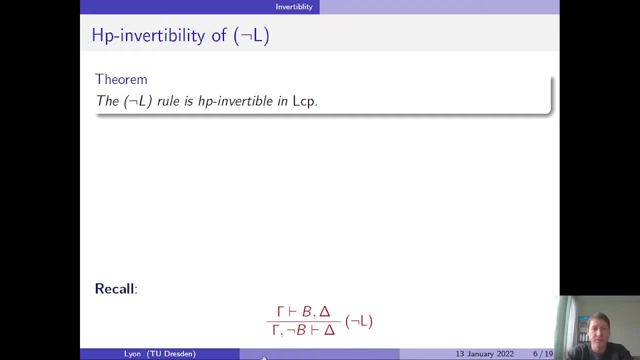 in our sequent calculus. So let's go through the proof of that claim Now. just as a reminder, the negation left rule is of the following form: It says that if I have a sequent which is derivable and has a formula B on the right-hand side, 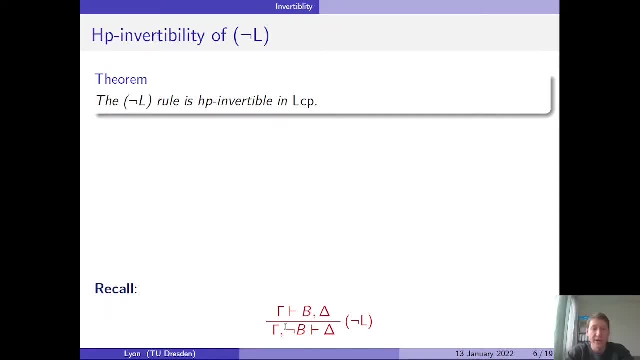 I can flip it over to the left-hand side of the sequent so long as I introduce a negation in the process. And now what we're going to do is prove the invertibility of this by induction on the height of the given derivation. 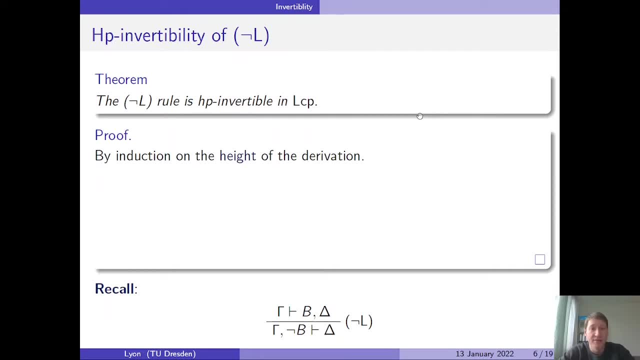 As I mentioned in the previous talk, the height of a derivation is essentially the length of the longest path inside of a proof. So a proof is as a tree-like structure And if you look at each of the paths throughout that tree-like structure, 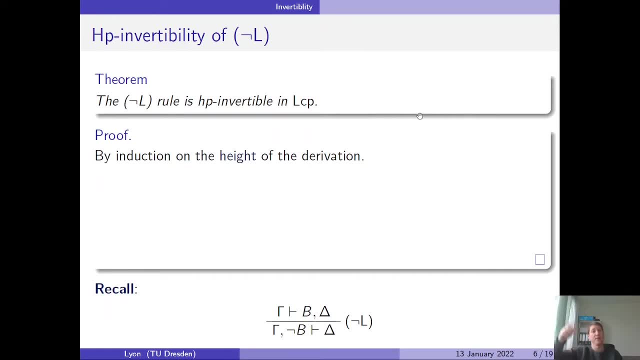 and you calculate how many sequents exist along those paths, the maximum number among all of those numbers will be the height of the derivation, And this is used quite often in proving results in proof theory. is this notion of the height of a proof? 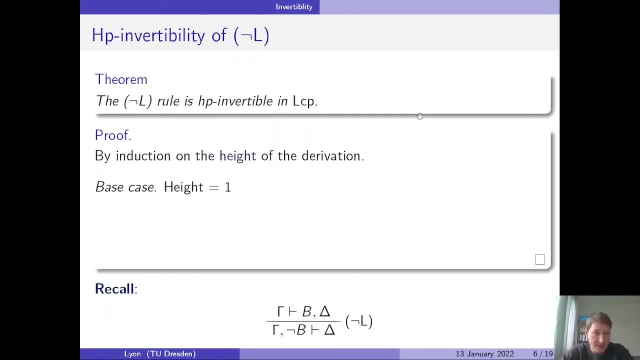 So we're going to use that here And now. in the base case, we assume that the height of our derivation is 1. Well, this must mean that our sequent that was derived is derived by means of the axiom rule. where we have a sequent, 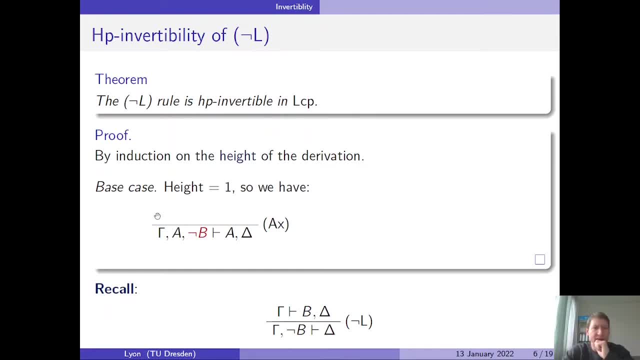 Now observe that the sequent obtained by the axiom rule is an instance of the conclusion of the negation left rule. Why is that the case? Well, on the left-hand side of the sequent occurs a negated formula, namely not B. 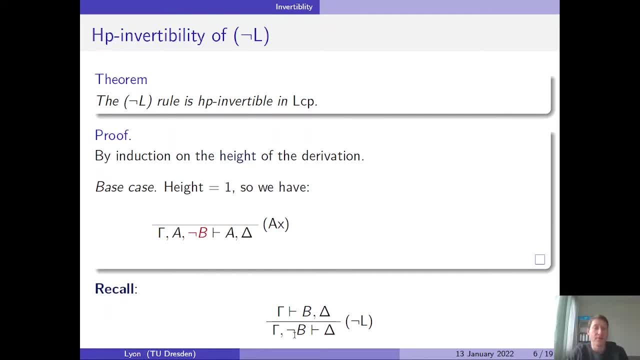 And now the question is: can we come up with a proof in our sequent calculus for classical propositional logic where instead of having a not B on the left, we have a, B on the right-hand side? Well, it's quite easy to see that this would also be another instance of the axiom rule. 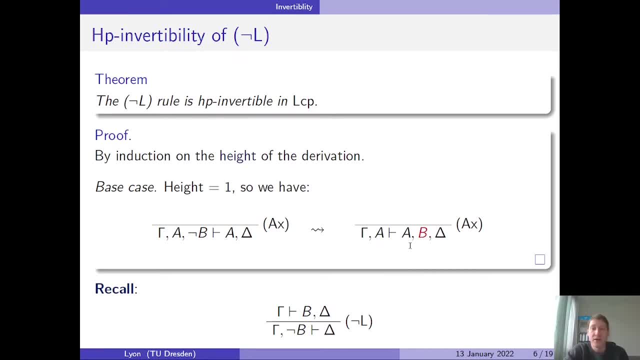 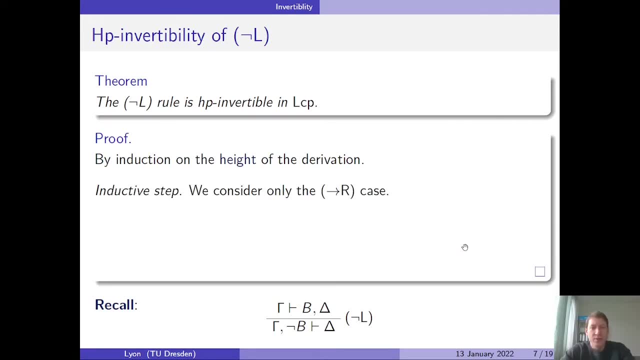 because we have this A occurring on the left and on the right. So that covers the base case. Let's now move on to the inductive step. So in the inductive step we're only going to consider the case where the last rule applied is the implication right rule. 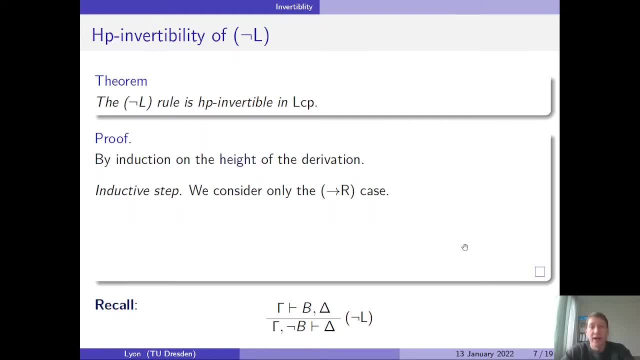 Now this is typically how proofs go In proof theory: you prove the result by induction on the height of your derivation and then you make a case distinction based on the last rule that's applied in the proof that you're analyzing. So here the last rule, we're assuming is the implication right rule. 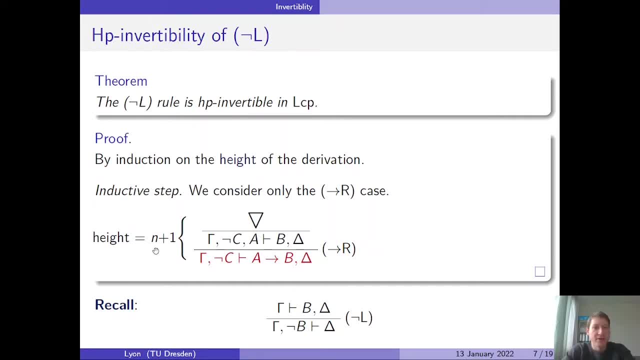 And now we assume that the height of the given derivation is a height n plus 1, and this little triangle here just indicates that there is some proof above that. Now notice that the conclusion of this is an instance of the conclusion of the negation left rule. 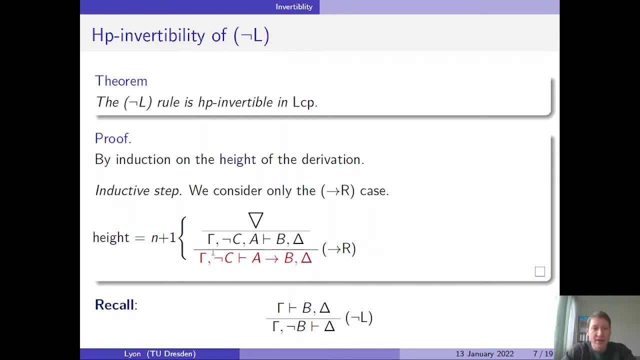 Why is that the case? Because there is a, not C, occurring on the left of the sequent. In other words, there is a negated formula which occurs on the left of the sequent. And now our goal is to show that we can derive essentially the same sequent with the same height or less. 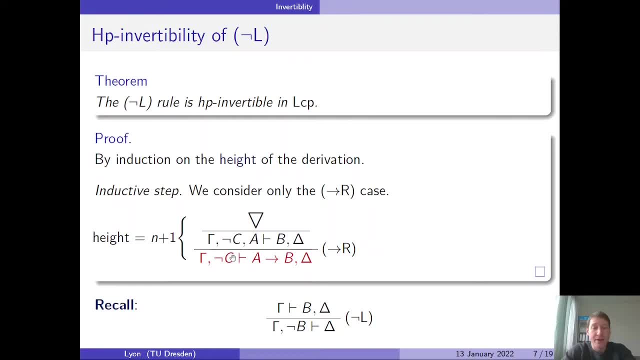 but where, instead of having a, not C, on the left, we have a C on the right, which would be an instance of the premise of the negation left rule. So how can we show that? Well, if we observe the premise of the implication right rule, it is of height n. 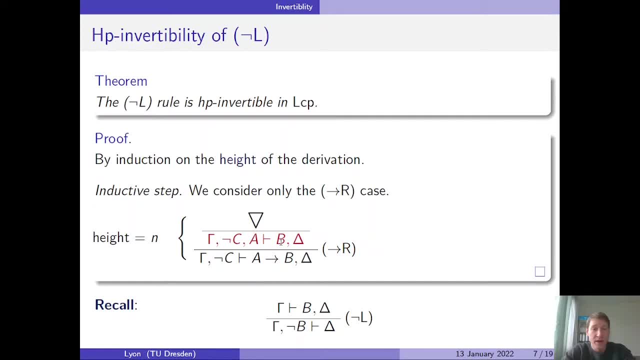 and it's one higher than this given derivation And therefore we can invoke the induction hypothesis or inductive hypothesis to derive the same sequent, but instead, where we have a, not C, on the left-hand side, we have a C on the right-hand side. 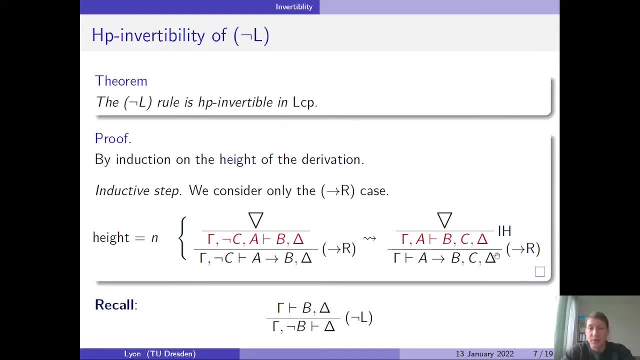 And now what we can do next is apply the implication right rule to this to obtain the desired sequent. So we have a proof of an instance of the premise where this, not C, has been moved to the right and the negation has been stripped off of it. 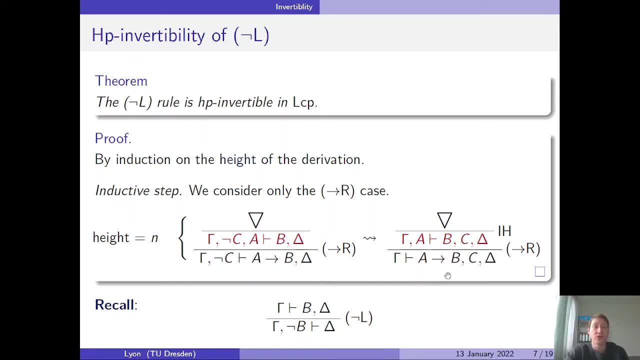 So this gives an idea about how HP invertibility is shown in general. Of course, to finish this proof, you would also have to consider the negation left case, the negation right case and also the implication left case as well. Let's now move on to cut elimination. 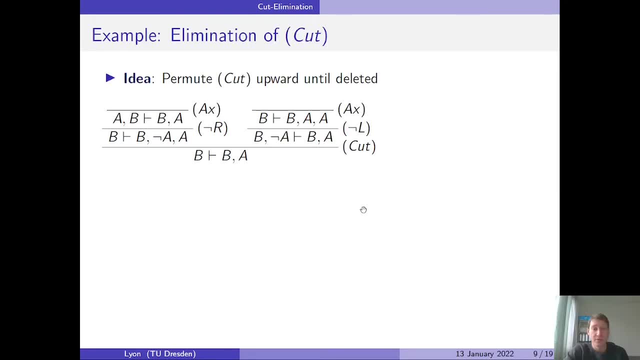 which is a very famous topic in proof theory. Now, before I go on to explain how cut can be eliminated in general from our given sequence system, what I'm going to do is give an example of how cut is permuted upwards in a proof. 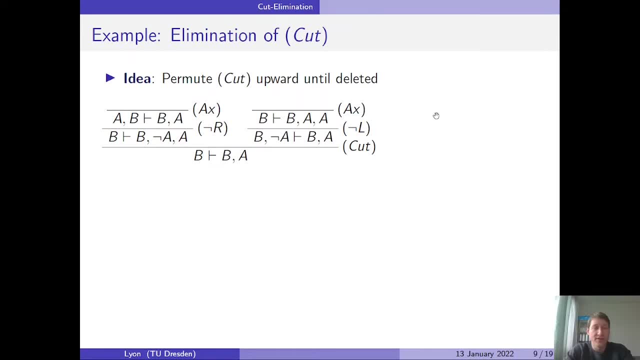 until it is deleted at the axioms. So let's look at this particular derivation that we're given and I'll explain how cut can be deleted in a very methodical fashion. So observe that the, not A, is the cut formula occurring in the left premise and the right premise here. 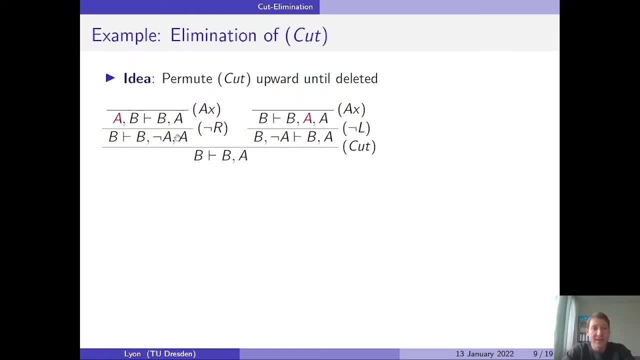 And we can observe or we can see that the not As were obtained were our principal formulae, that are obtained from the auxiliary formulae A occurring in the premise of the not right rule and the premise of the not left rule. In other words, looking at the not right rule. 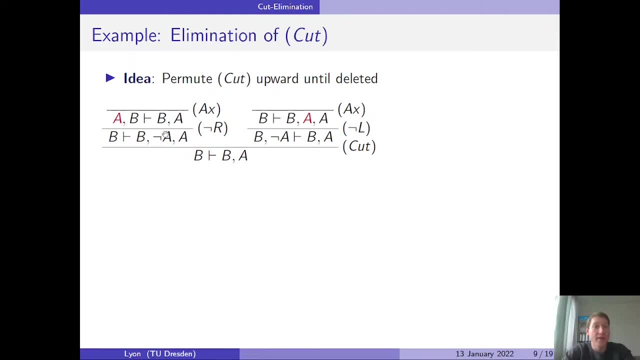 this A was used to apply the not right rule and introduce the not A cut formula, occurring in its conclusion and in a similar fashion with the right premise of cut. But now, if we look at these two sequences, this one has an A on the right and this one has an A on the left. 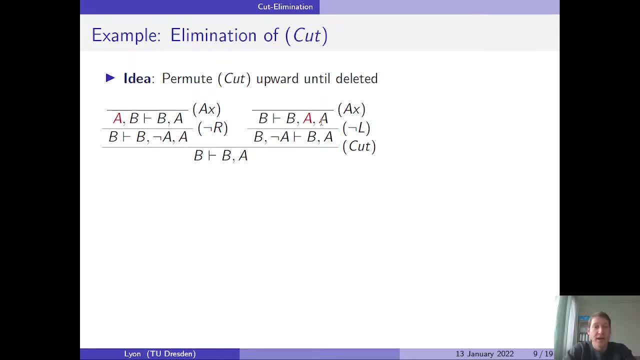 and the contexts aside from that formula match, and so, therefore, we can actually apply cut to each of these axiom instances, giving this derivation where the cut has essentially been moved upwards. Well now, if we look at the conclusion of this proof, it turns out that it is an instance of the axiom rule as well. 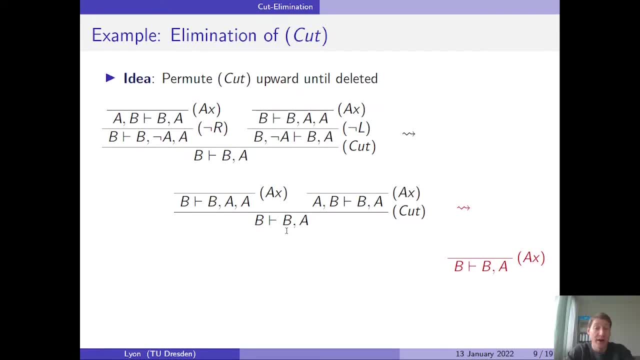 because there's a formula B which occurs on the left and the right hand side. Now, although we can see that this concluding sequence here in the given proof is an instance of the axiom rule, what this example shows is how cut elimination works, how it gets moved upwards in a proof. 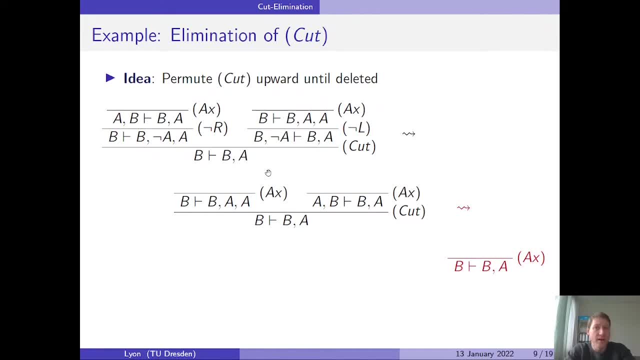 Now there are things which are sort of reduced through this process which we use to establish that this process of eliminating cut will always eventually terminate. So the first thing which decreases or could decrease when moving a cut upwards is the complexity of the cut formula. 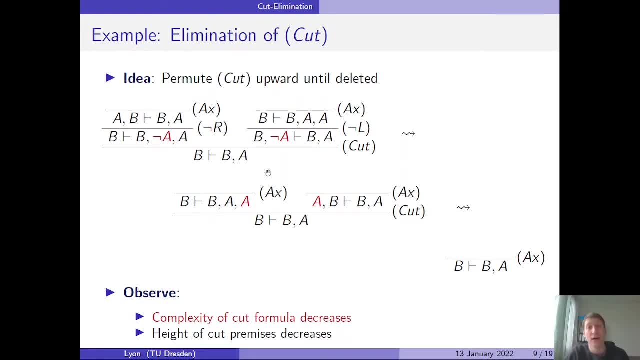 namely the number of logical connectives which occur in the cut formula. So if we look at this particular example, we have a, not A, as our cut formula. in our given derivation and in the second proof we used A instead of not A. 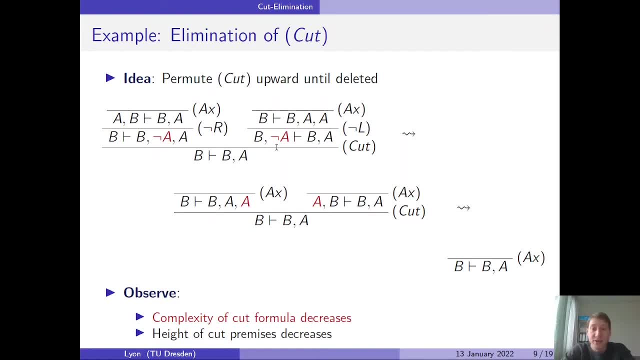 which has a lower complexity because it does not have that negation prefix to it. So that's the first thing which can decrease through cut elimination and which we use to our advantage to establish the elimination of cut, the complexity of the cut formula. And the second is the height of the cut premises. 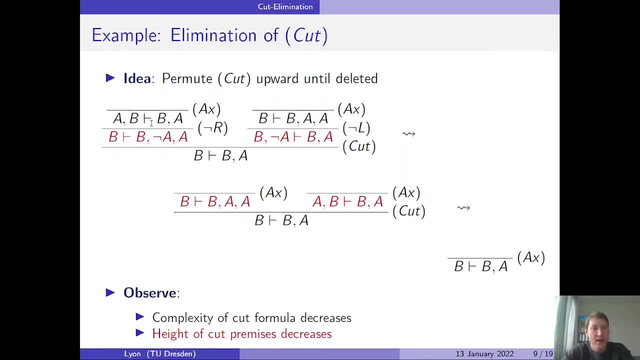 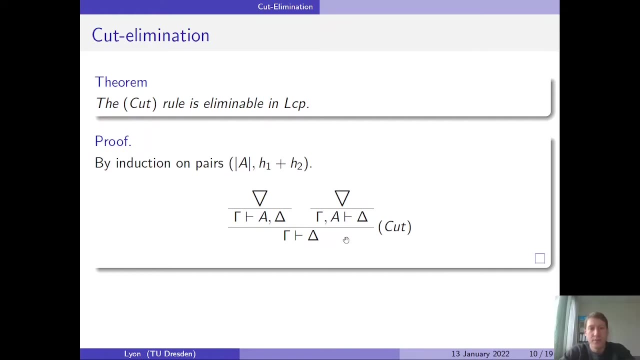 So notice here that the premises of cut in the given derivation have a height of 2.. Now in the second obtained proof each has a height of 1. So we notice that the height of the cut premises has decreased as well. Now, using these things, we're going to show or argue. 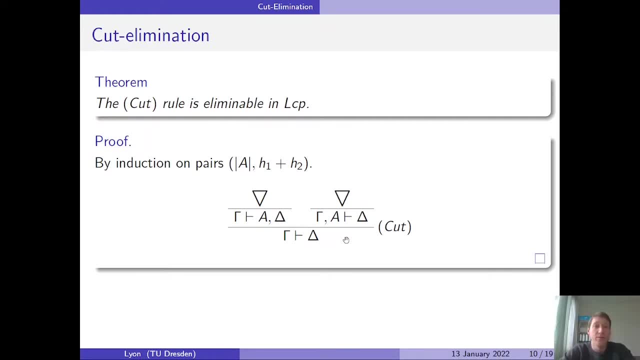 we'll only look at a few cases, but it should get the idea across that the cut rule is eliminable in the sequence calculus for classical propositional logic, namely LCP. So how are we going to show this? Well, we're going to prove the result by induction. 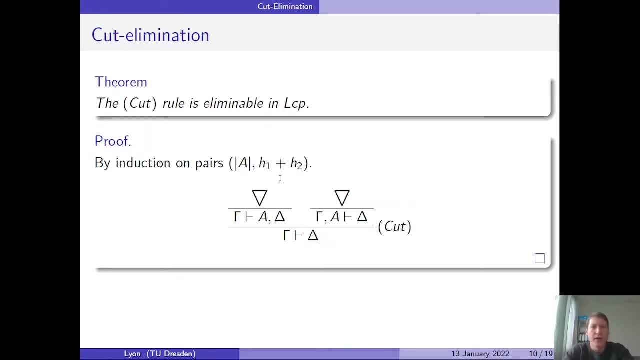 of pairs of the following form, where we are doing induction based on the lexicographical ordering of these pairs. So what is the first component of the pair? The first component of our pair is the complexity of the cut formula, namely the number of logical connectives that it possesses or contains. 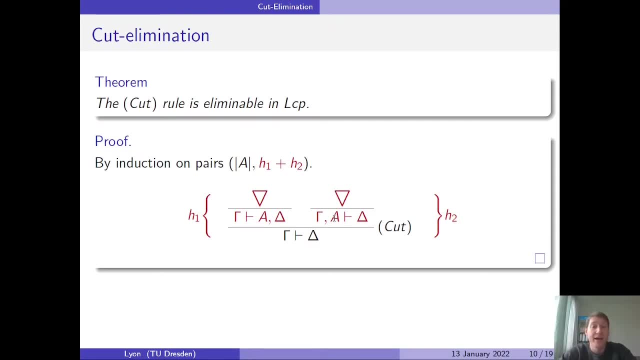 And the second component of the pair is the sum of the heights of the derivations of the premises of cut. So the left premise of cut here is shown to have a derivation height of h1, and the right premise of cut has a derivation of height h2.. 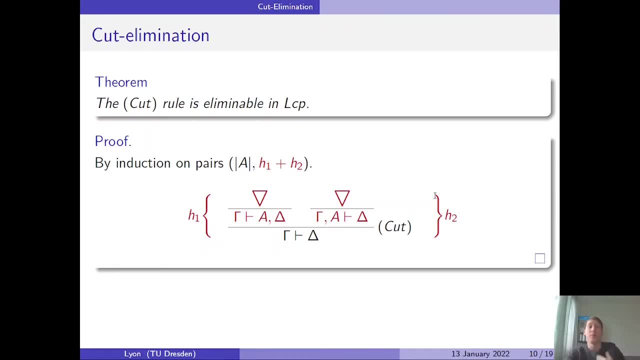 So again we're going to show that cut is eliminable by induction on the lexicographical ordering of these pairs. Okay, So now let's look at one case. Remember there's a lot of different cases that pop up in cut elimination. 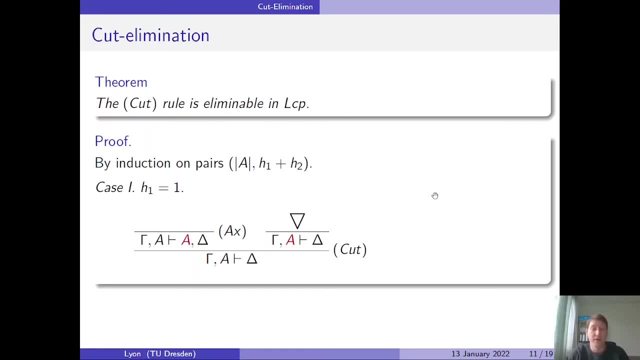 that you have to analyze. We're only going to analyze a few, but it should get the idea across to the viewer. So in the first case, let's assume that h1 is 1.. In other words, the height of the derivation of the left premise of cut is 1.. 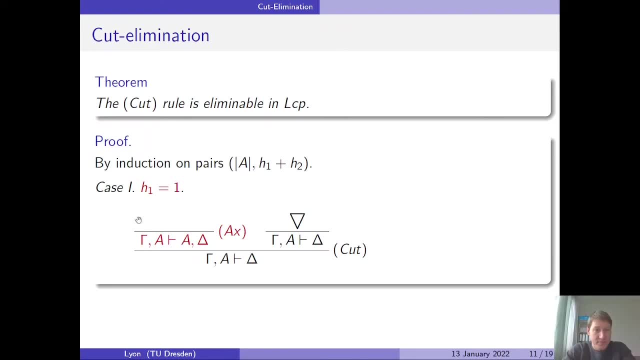 Now, in that case the left premise of cut must be an instance of the axiom rule. We're also assuming that the cut formula A is principled in that axiom. Now, in this case we have that this is the left premise of cut. 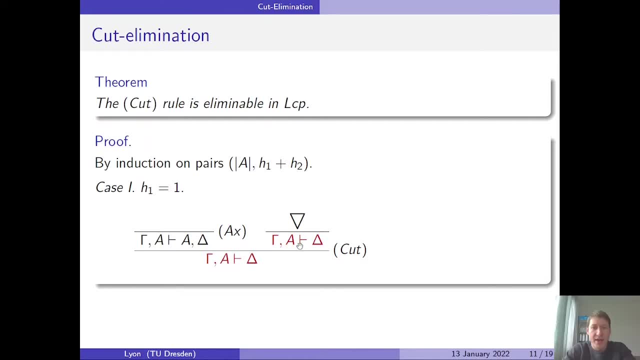 and we have that this is the right premise of cut- gamma, A, sequent arrow, delta, And we can see that the conclusion of cut is the same or identical to its right premise, And what that means is that we can eliminate cut by simply just taking the derivation. 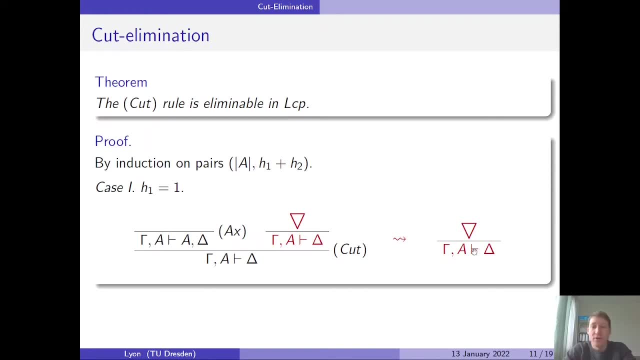 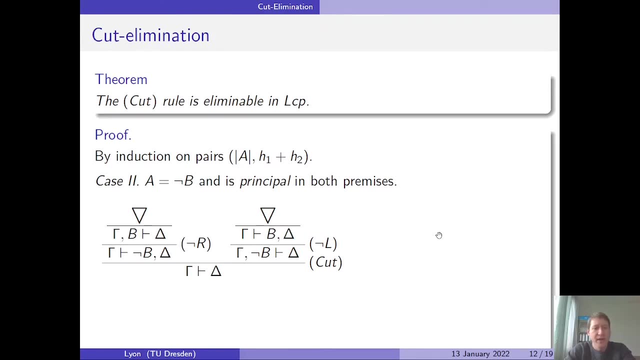 which gives rise to the right premise of cut. And now cut is no longer occurring here. So that's how this case is resolved. Let's look at another case. In this case, we're going to assume that the cut formula is not B. 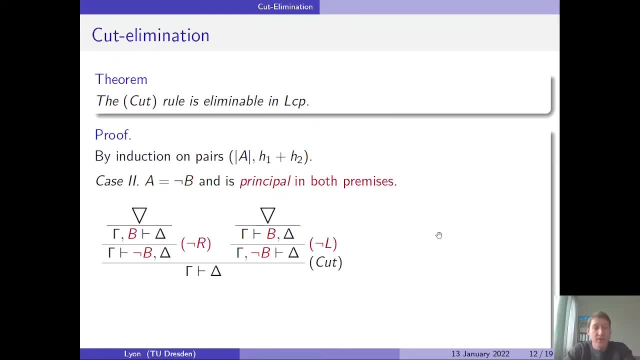 so it's a negated formula And we're going to assume that the cut formula is principled in both premises of this instance of cut or this use of cut. What this means is that both of the rules that are used to give rise to the premises of cut 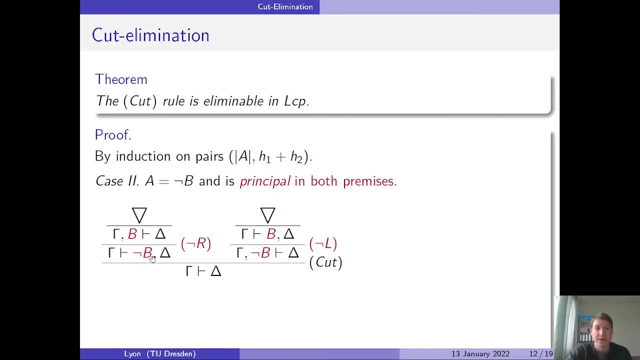 introduced that cut formula, in this case being not B. So in the left premise we had that not B was introduced by the negation right rule and in the right premise of cut we had that not B was introduced by the negation left rule. 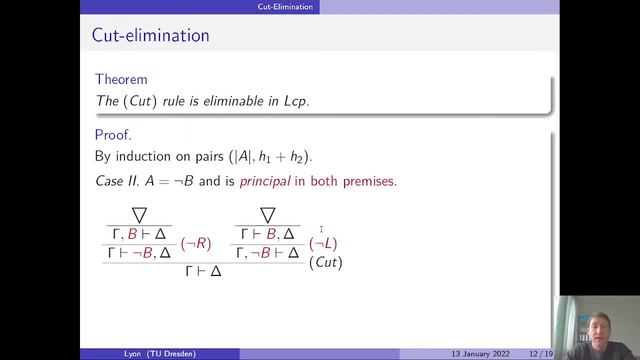 And now what I'm going to do is show you how we can move the cut upwards in this case. So if we observe the premise of the negation right rule and the premise of the negation left rule, we can see that in the premise of negation right rule, 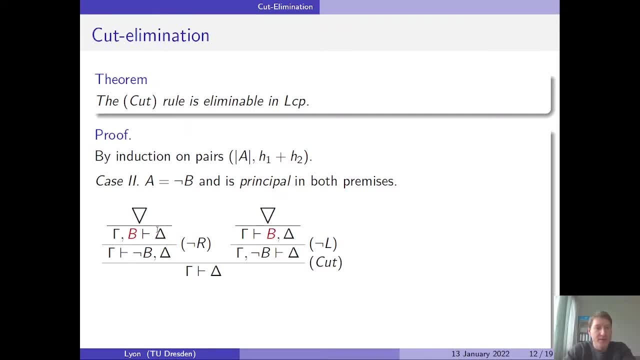 the premise of negation left, we have a B on the right. In the premise of the negation right rule, we have a B on the left And the context, gamma and delta or the side formula, are identical to each other. 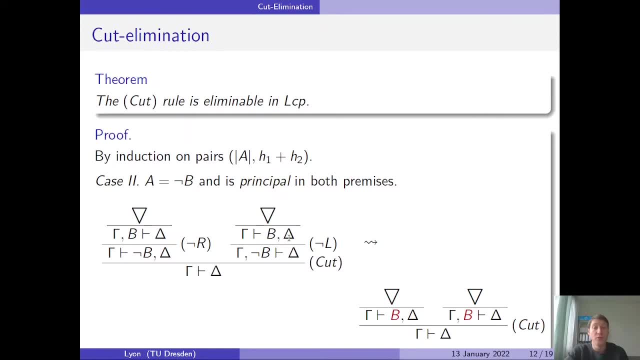 What this means is that we can apply the cut rule to these premises of these negation rules. We can cut on B instead of not B. Now, in this case, what has happened is the complexity of the cut formula has decreased because we're cutting on B as opposed to not B. 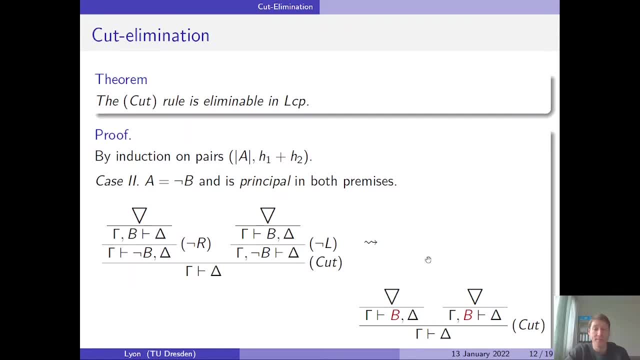 And also, at the same time, the heights have decreased. Alright, let's look at another case showing how to eliminate cut. So here we're going to assume that our cut formula is an implication of the form B implies C. We're going to assume that it is principal in the left of cut. 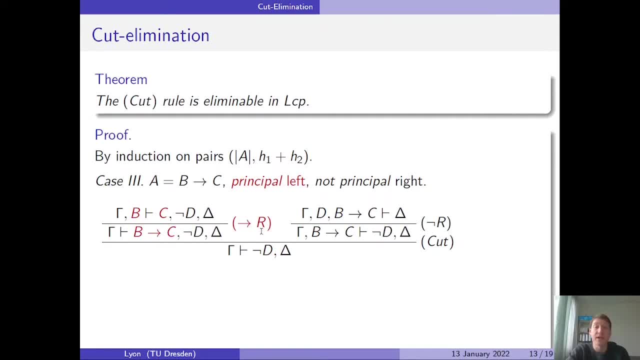 meaning it was introduced by the implication right rule And we're going to assume that it is not principal in the right premise of cut. So we're going to assume that some rule, in this case it's going to be the negation right rule. 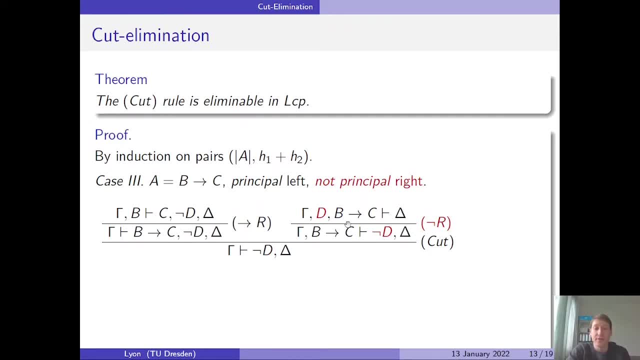 was applied to give rise to the right premise of cut, introducing this negated D, which occurs in the succeeded or consequent of the right premise of cut. Okay, so this is the situation we're going to analyze Now, if we look at the left premise of cut and we look at the premise of the negation right rule. 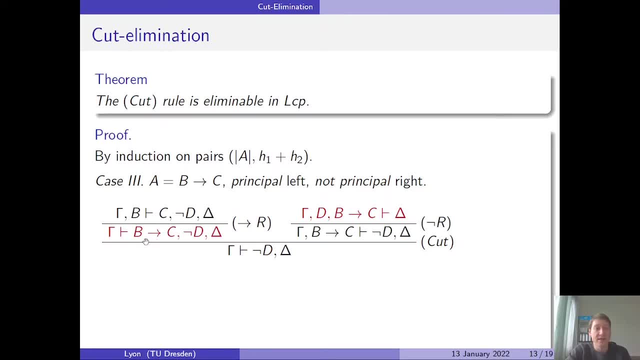 we can see that the left premise of cut has a- B implies C in its consequent or succeeded, And in the premise of the negation right rule we have a- B implies C in the antecedent. So now these sequence are rather similar. 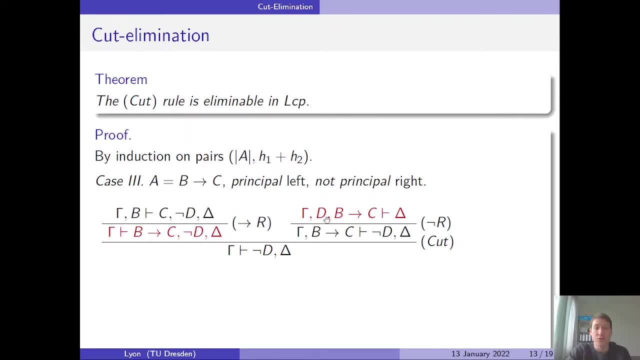 The only difference between them is that the left premise of cut has a, not B, in the conclusion and the premise of negation right has a, D in the antecedent, And so, if we're able to rectify this so that the contexts match, 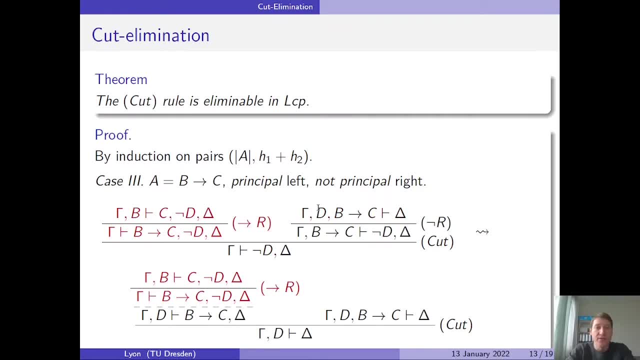 we can cut on. the B implies C. And now this is how we're going to do that. First we take the derivation giving rise to the left premise of cut, and then we take the derivation giving rise to the premise of negation. right rule. 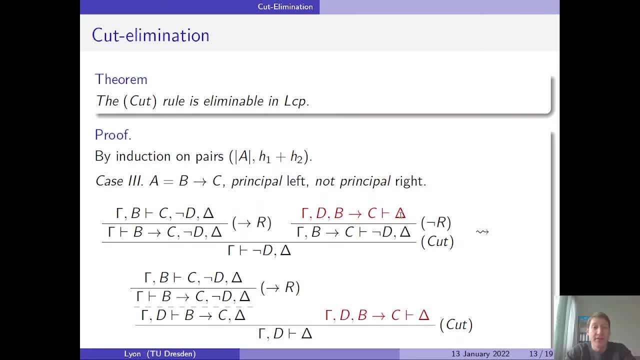 So observe that this derivation will be of height h2 minus 1,, since we're assuming that the right premise of cut was derived with a height of h2, and this is 1 higher than the previous. And now we can invoke the HP invertibility of the negation right rule. 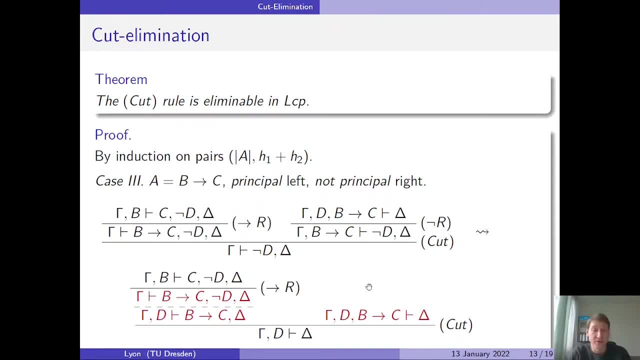 which is something that we covered in the previous section of this talk. So if we look at the sequence that's derived with the implication right rule, I have a, not D, occurring on the right-hand side of the sequence Now, since I know that the negation right rule. 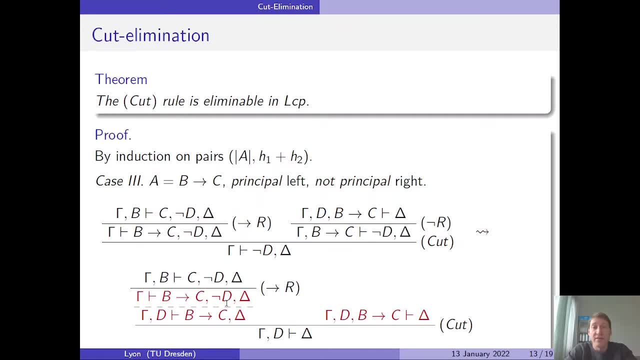 is height-preserving invertible. I have a derivation whose height is, at most, h1, but where, instead of a not D being on the right-hand side of the sequence, I have a D on the left-hand side of the sequence, And now, by making use of that result, 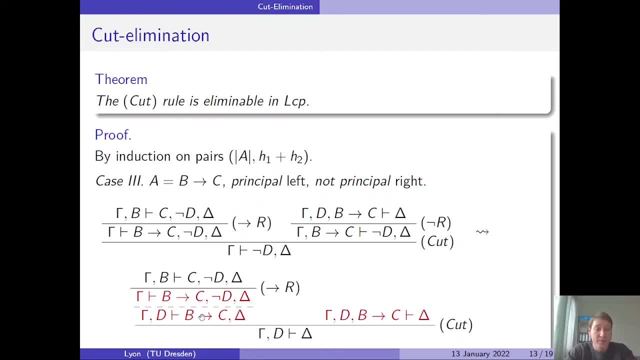 I have obtained a proof of gamma D sequence arrow. B implies C delta and I already know that I have a derivation of gamma D. B implies C sequence arrow delta and I can cut on this. B implies C yielding the sequence gamma D sequence arrow delta. 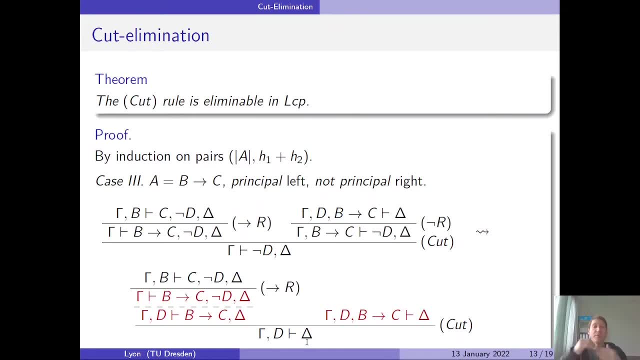 Now the conclusion that I need remember: when I move the cut upwards, I need to show that the cut is moved higher in the derivation and the same sequence is derived, And so I can move the cut upwards and derive the same thing If we compare the conclusion to the originally given. 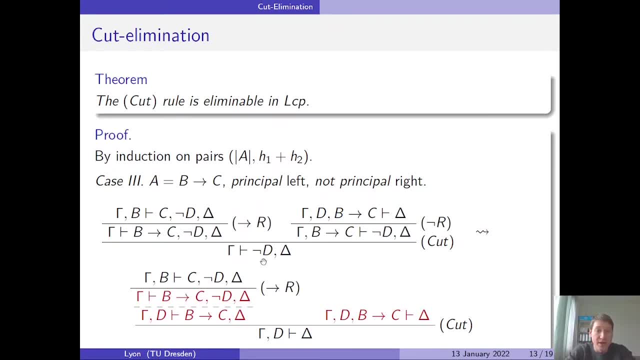 in the originally given derivation we have a, not D, on the right-hand side. Here we have a D on the left-hand side. So what can we do? We can apply the negation right rule and move this D to the right. 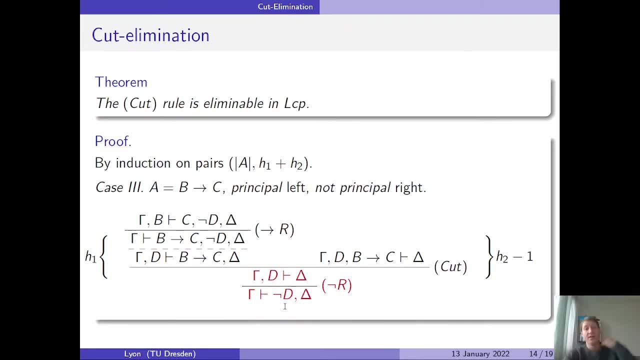 and reduce any negation. Do so Now. observe that the complexity of the cut formula. B implies C is exactly the same, so that it has not been reduced, but the heights, the sum of the heights, has been reduced by 1,. 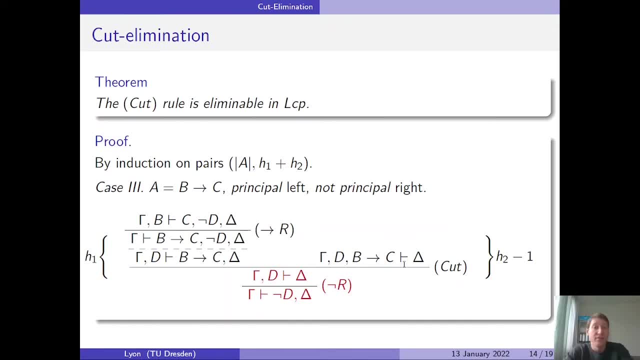 because now the right-premise of cut has a derivation whose height is h2-1,, as I mentioned previously. So we've moved or shifted the pair that we're using in this type of cut farther down in the lexicographical ordering. So we're allowed to. 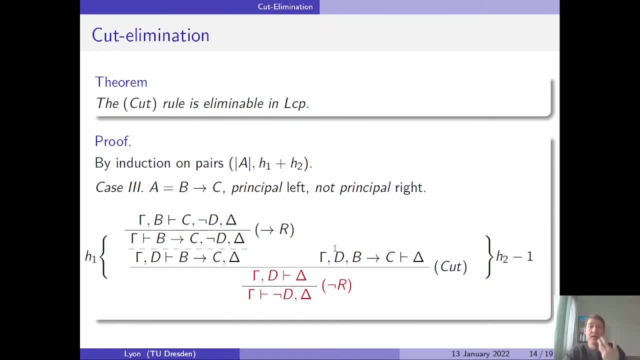 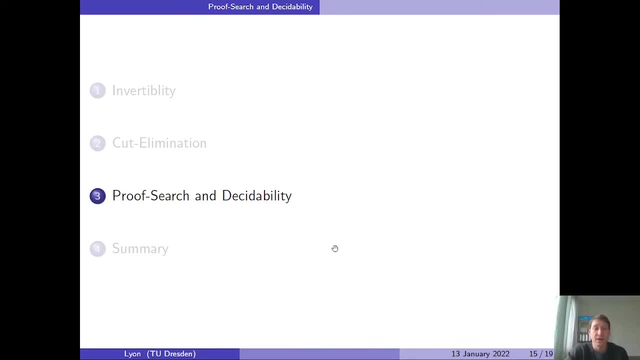 it shows that this cut process will terminate. since this is a smaller pair is associated with this cut. Okay, so now let's look at the consequence of cut elimination. Now, in the first talk, I defined LCP, which is the sequent calculus I've introduced. 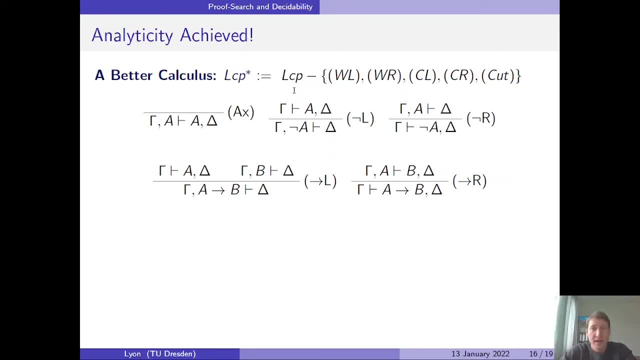 for classical propositional logic And that sequent calculus contained five structural rules, Weakening rules, contraction rules and also the cut rule. So now we can affect effectively, through our admissibility, results of the weakening and contraction rules discussed in the first talk. 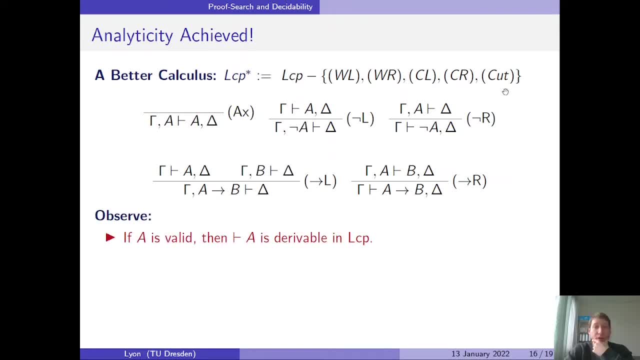 and cut elimination shown here, we can obtain a new calculus where a fragment of LCP called LCP star, which just consists of the four logical rules for negation and implication and also the axiom rule, And we know that this calculus is complete. 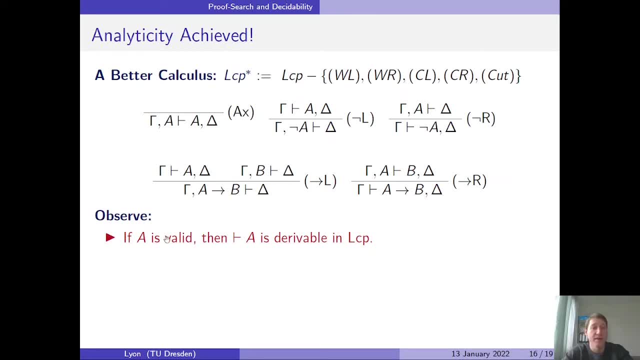 for the following reason: In the previous talk we argued or showed that if some formula was a validity in classical propositional logic then it was derivable in LCP, so in the calculus with the structural rules. But now we've shown that all the structural rules 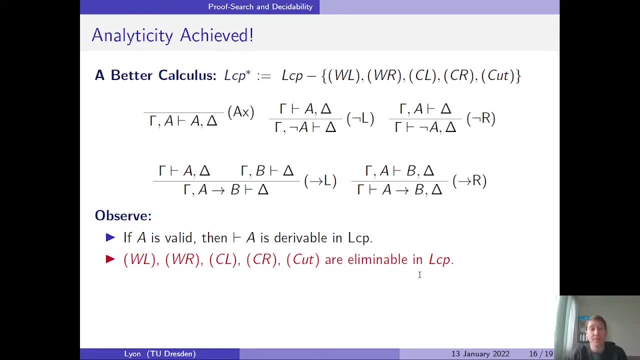 are limitable in LCP. In other words, anything which can be derived with them can be derived without them. That means that if you give me a validity of classical propositional logic, I can derive it in LCP. and due to this second fact, 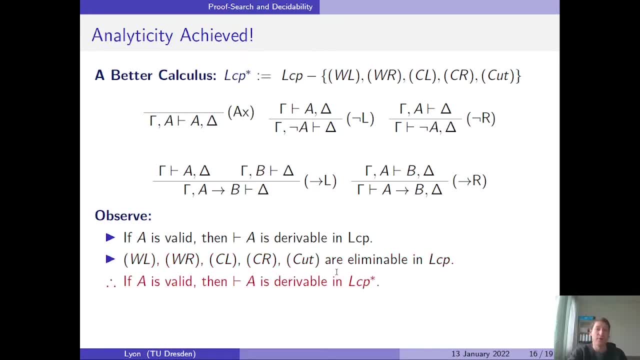 I can derive it without any of the structural rules. Therefore it will be derivable in this new calculus, LCP star, this more refined calculus. And what's nice is that just by observing the logical rules of this calculus we can determine that classical propositional logic. 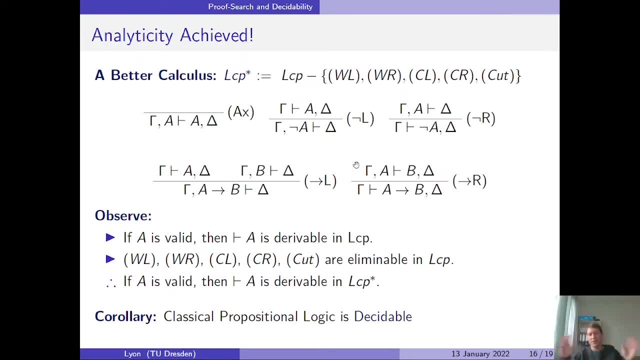 is decidable. Now, it's well known that classical propositional logic is decidable, so what should be emphasized here is not the decidability of this particular logic, but the methodology that was used in recognizing this fact. So you could have a. 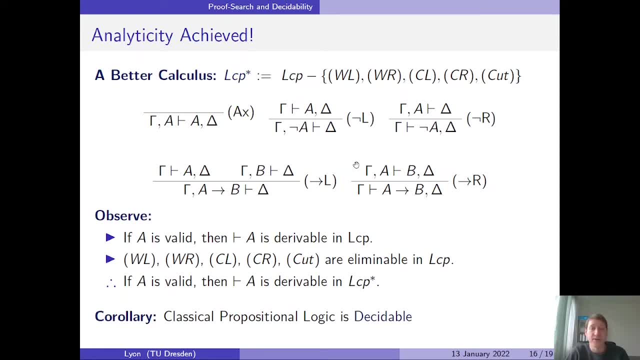 let's say sequence calculus for a more complicated logic or for a different logic, For example say intuitionistic propositional logic, whose calculus is not very different than the one presented here for its classical version. And just by going through this process, 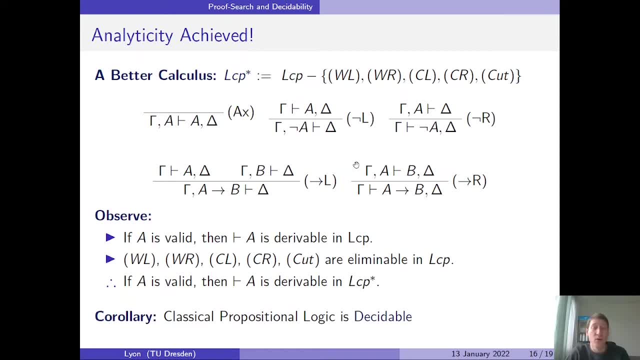 of eliminating the structural rules and doing culmination, one can come to the same conclusion that the logic is decidable by looking at the calculus that is obtained. after all, structural rules are removed. Now what I'm going to do is try to explain how, looking at these rules, 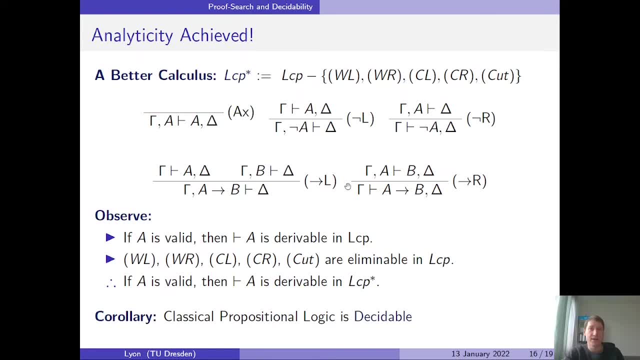 tells you that your logic is decidable. So I've written on the top of the slide analyticity achieved. Now, analyticity is not a rigorously defined notion in proof theory, but typically what we mean when we say that a proof system is analytic. 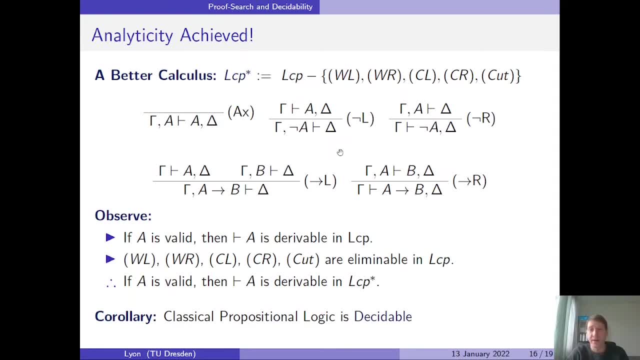 is that it has the subform property or some variant For this talk. we're going to say that analyticity means the same thing as the subformula property, but it does take on different versions in the literature. What is the subformula property? 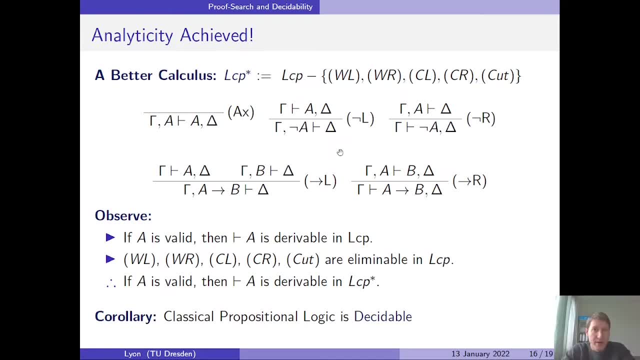 Well, calculus has the subformula property when all the formulae used in the premise or premises of any rule are subformulae of those formulae which occur in the conclusion of the rule. We can see, for example, in the implication left rule: 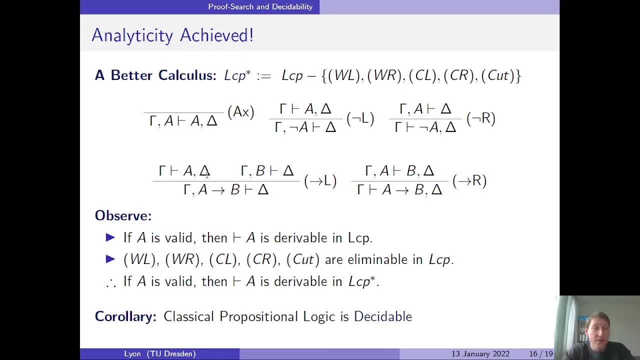 if we look at the left premise, of course the gammas and the deltas, the formulae which occur in these contexts are subformulae of themselves in gamma and delta. but A is a strict subformula of A implies B. Similarly, B is a strict subformula. 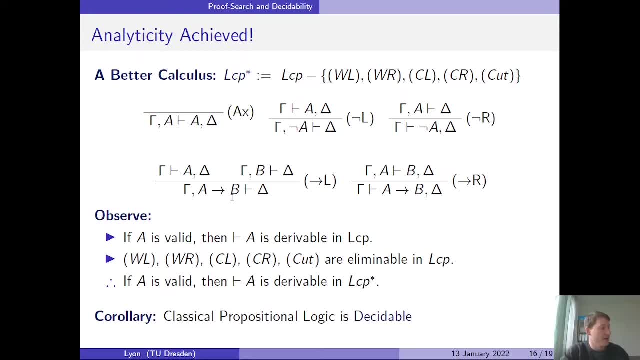 of A implies B, So we can see that the complexity of the premises is smaller than the complexity of the conclusion and that it only makes use of subformulae of the conclusion. So this is how we can recognize the citability for logic. 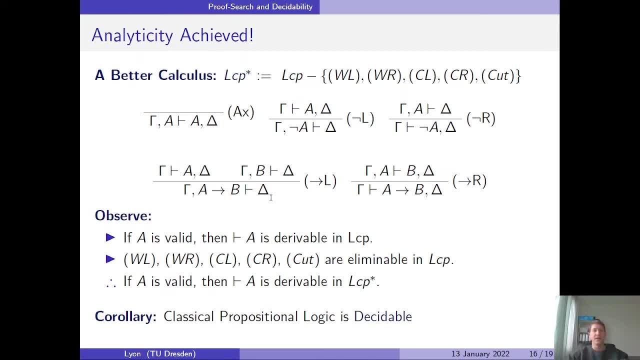 Give me a formula and I apply these inference rules, these ones shown here on the slide, in reverse on that formula. that process will eventually terminate, because every time I apply a rule in reverse I get a structure which is less complex, it has less logical connectives. 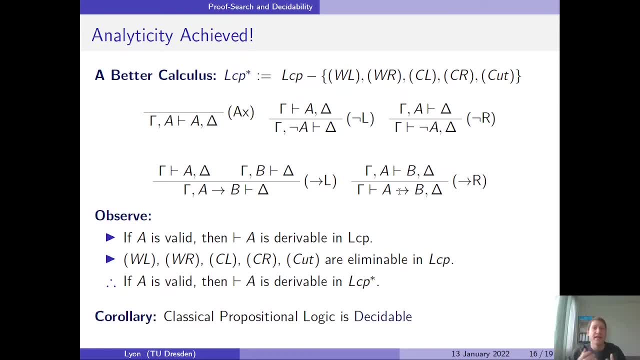 And so what this means is that there's only a finite number of proofs for any given provable formula. Now, if I know that there's only a finite number of proofs, what I can do is search throughout that finite space. so you give me a formula. 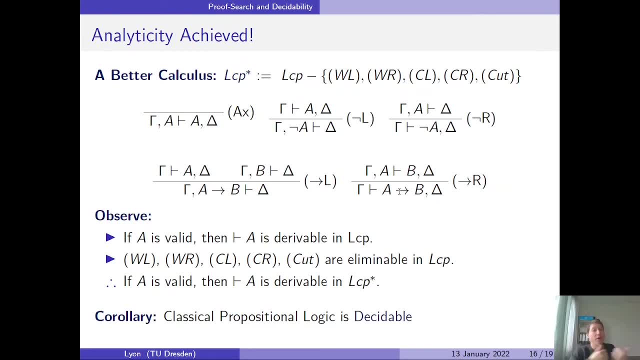 I search throughout that finite space. if I find a proof of it, I know it's valid because it's derivable. And if I can't find a proof of it, then I know it's invalid. So this is how you can use. 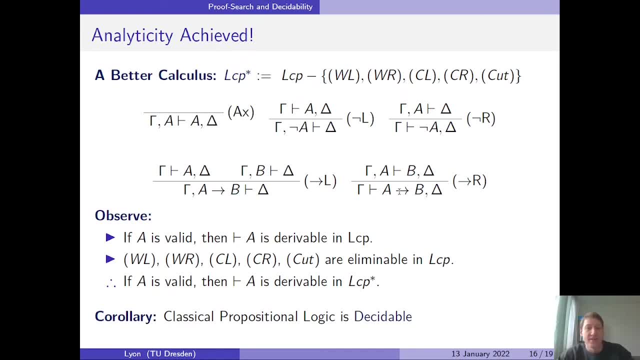 the subformula property to recognize that a logic is decidable. Now, here again, we know that classical propositional logic is decidable. very easy to give a decision procedure by making use of standard truth tables. but this is another way of recognizing it. 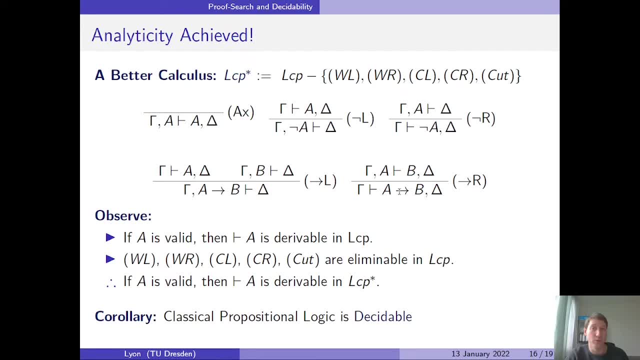 by just looking at the structure, The inference rules and its corresponding sequence calculus. And this can be done for different kinds of logics, substructural logics or modal logics, for example. Okay, so now I've explained that just by looking at the structure of the rules. 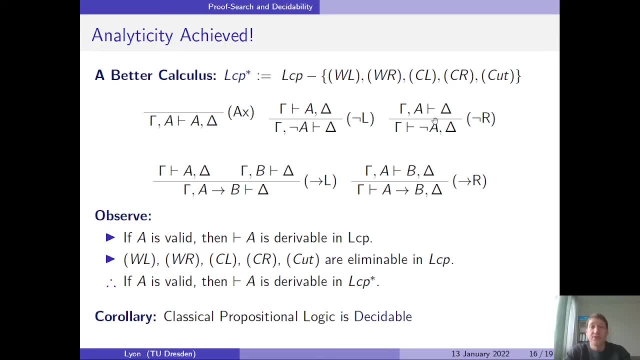 just because this new calculus we obtained after eliminating our structural rules has the subformula property that our logic is decidable. but knowing that a logic is decidable is different than actually writing a decision procedure for the logic, And this is where a proof search comes in. 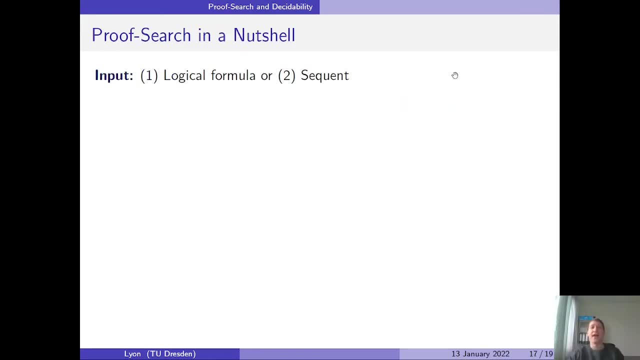 Proof search is essentially a strategy for establishing the decidability of a logic, And I'm going to go over it on this slide. So let's quickly go over proof search. How does it work? You give me a logical formula or you give me a sequence. 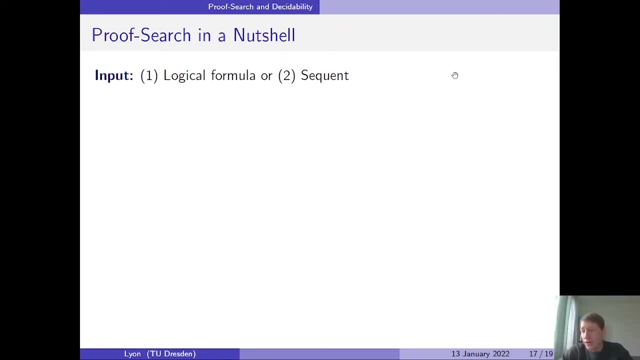 Depending on your proof search algorithm or the logic that you're dealing with, you might want to take one or the other as input. In this case, we're going to take sequence as input. Now what you do is you apply the rules from your calculus. 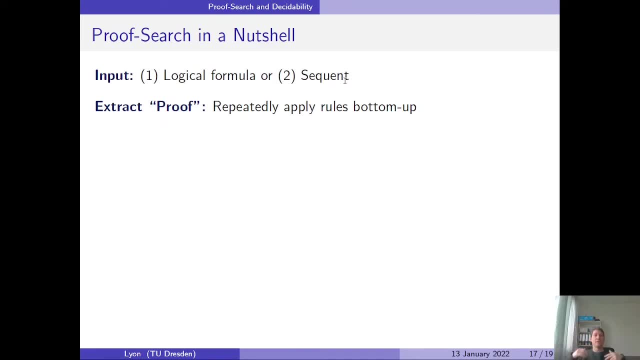 bottom up over and over again to extract a proof. Now, I put proof- this word in quotation marks here- because what you might obtain in the end is something that is either is an actual proof in your calculus, or you might obtain something which 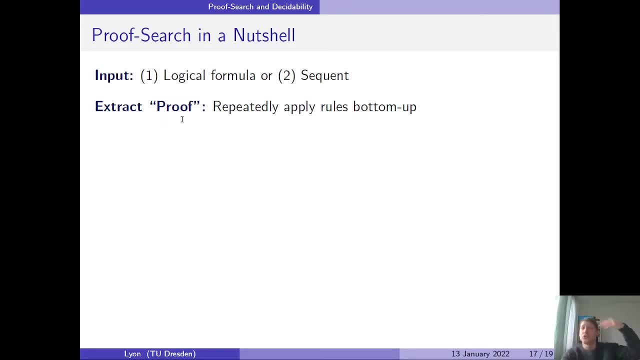 looks a lot like a proof, but the initial sequence in the proof, which should be axioms or not axioms, And you can actually use those, as I'll show in just a moment, to construct a counter model of your input formula. 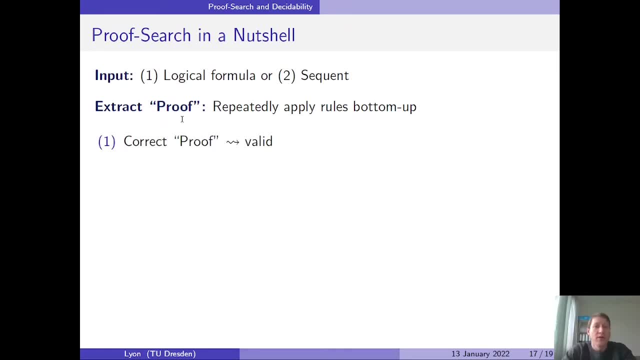 So let's go through how proof search works. So let's take a sequence as input and I'm going to show here the first case where we obtain a correct proof and why the input sequence is valid. So let's take this sequence as input and let's start applying rules from our calculus. 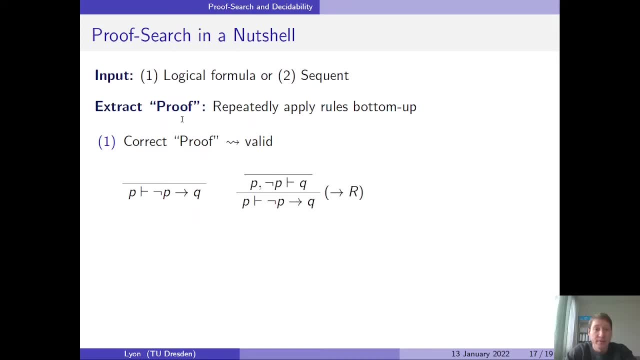 bottom up or in reverse to this given sequence. So first I apply the implication right rule. This puts the negation p on the left, It keeps the q on the right And now there's only one rule I can apply, which is the negation left rule. 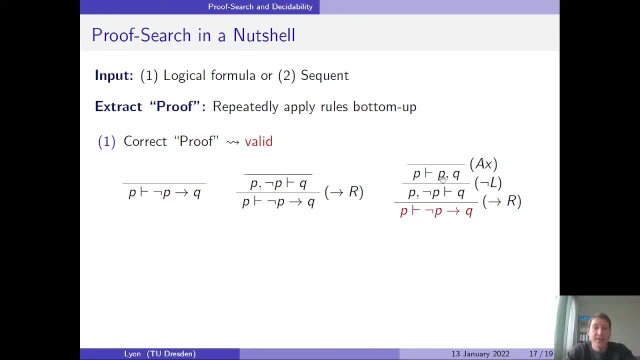 So I can take this- not p- and put it on the right, so long as I strip it of its negation. And now we can see that this is a proof witnessing the validity of the input sequence. We know that our calculus is sound, as mentioned in the previous talk. 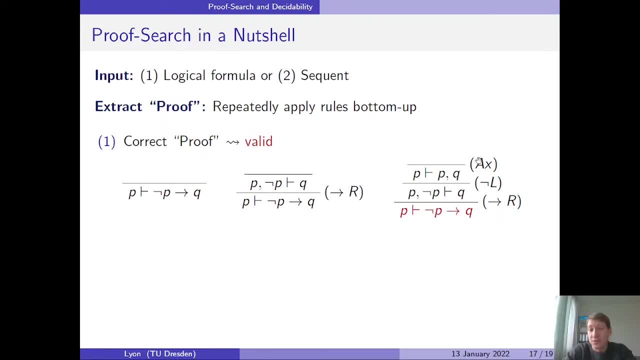 meaning anything which is derivable is valid. So since we have a proof in this calculus of this sequence, we know that the sequence is valid. Okay, let's look at what happens when our input is an invalid sequence. So here's an invalid sequence. 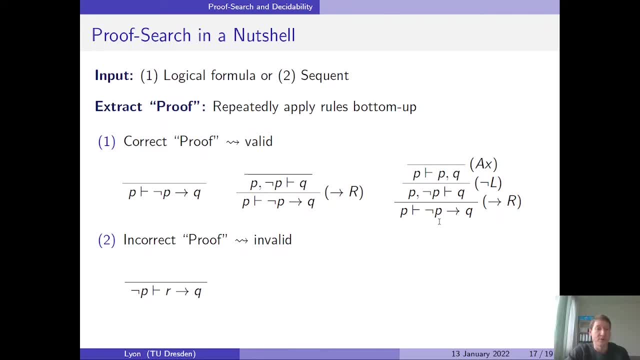 We don't know, say that it's invalid. yet We're doing proof search only once the algorithm is complete, So long as it is a correct terminating proof search procedure. do we then know that our sequence is valid, But this one's invalid, of course? 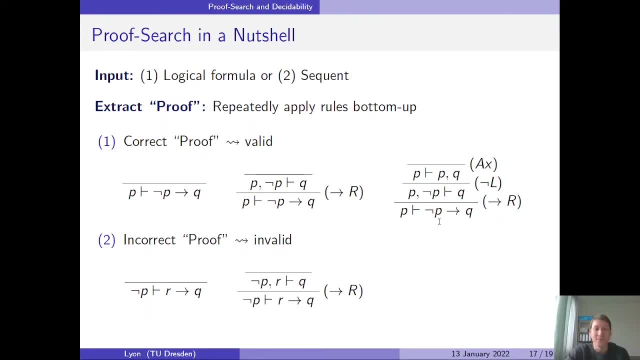 because we want to show an example of an invalid sequence. So again, I apply the implication right rule, first putting this r on the left-hand side, keeping the q on the right, And then I apply the negation left rule bottom-up. 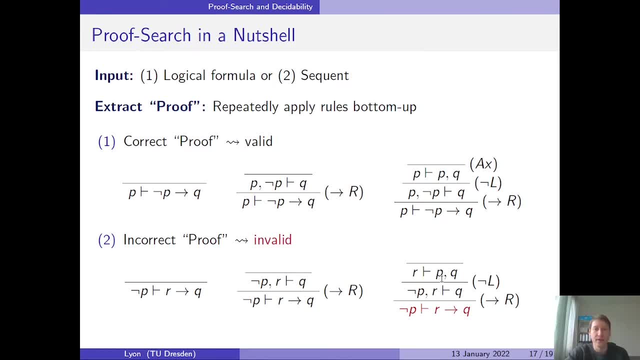 taking the p and putting it on the right. And now what's interesting is, this top sequence shown here can be used to define a counter-model for the conclusion of the proof. So remember that in classical propositional logic, our models or valuations, 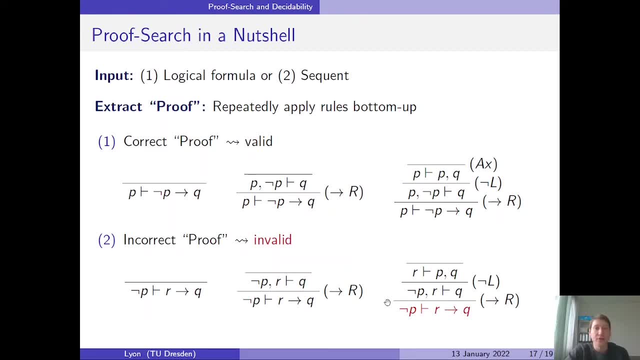 you might want to call them, assign truth values to propositional atoms in a formula, either one for true or one for false. So the way that we define a counter-model by making use of failed proof search, here is every propositional atom which occurs on the left of our sequence. 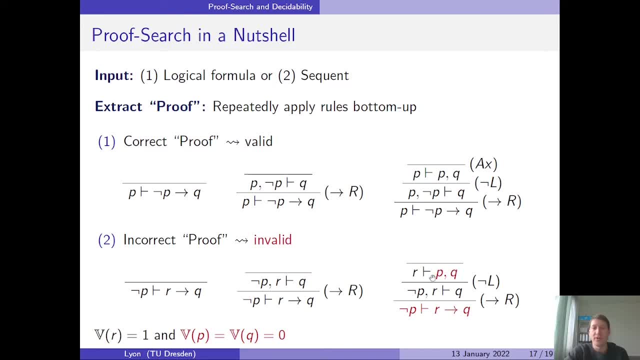 is assigned true and every propositional atom which occurs on the right-hand side is assigned false, namely p and q. But depending on the logic that you're dealing with and the type of data structures that are used in your sequence, it might be much less trivial. 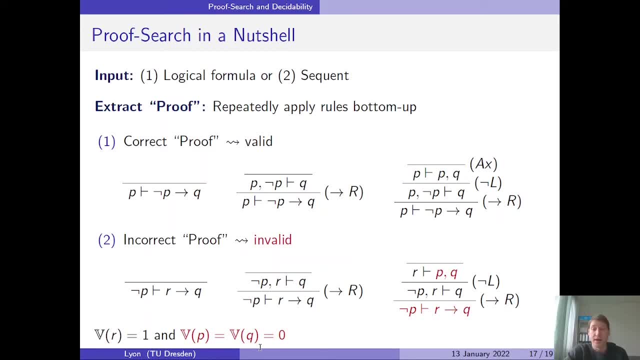 or much more complicated, to try to define a counter-model for your invalid sequence. Here it's relatively easy, because we're in the realm of classical propositional logic. So what's on the left becomes true and what's on the right becomes false. And now you can see that. 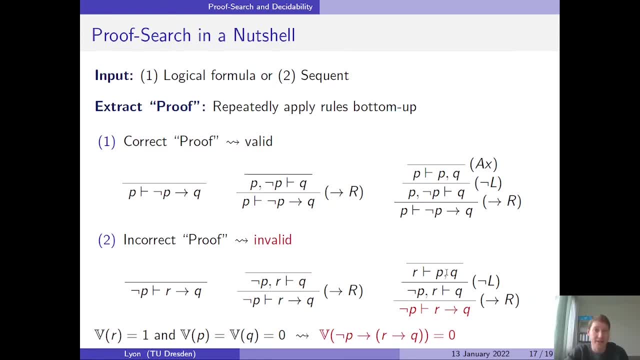 this valuation or this model invalidates the concluding sequence. Remember that a sequence is valid if, and only if, its formula interpretation is valid. So here's the formula interpretation of that concluding sequence. Now we can see that, because p is false, not p is true. 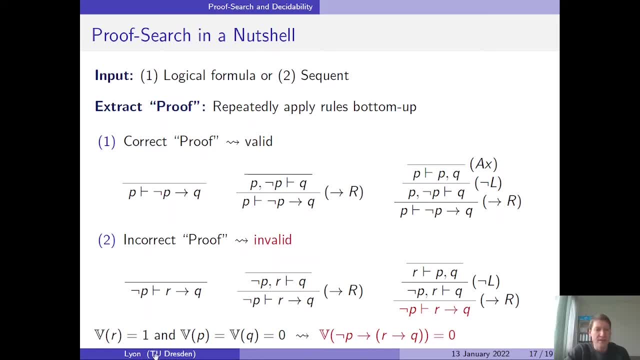 so we know that the antecedent of our implication is true. And since r is true and q is false, the conclusion, which is this implication here r implies q is also false. So we have something true implying something false by the truth tables. 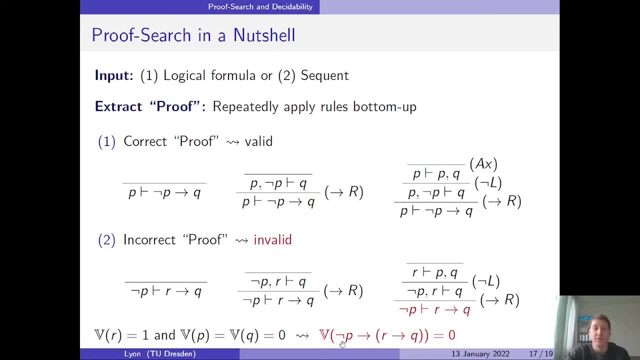 for classical propositional logic. We know that this formula is therefore false. So this is how proof of search works: You take a sequent or a formula's input. you apply the rules of your calculus in reverse If what you obtain is a proof. 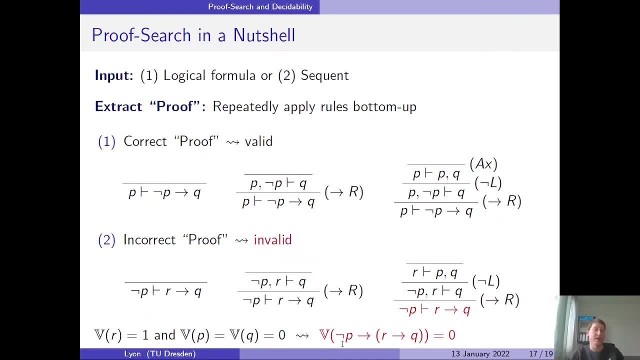 you know, the formula is valid And so long as your calculus has nice properties. if you obtain an incorrect proof, you can extract a countermole witnessing the invalidity of your input. So this is one way that you can write decision procedures for logics. 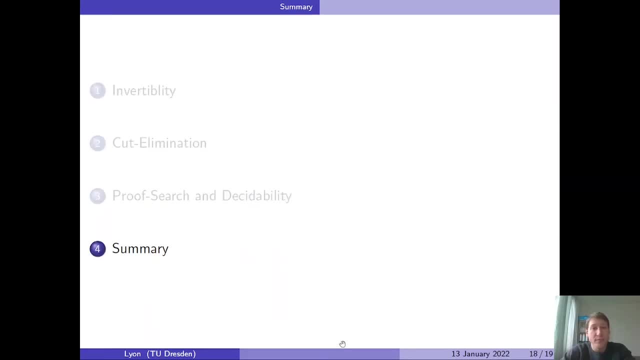 by making use of their sequence systems. Okay, just a quick summary regarding what we went over, and then the talk will be complete. So at the beginning I discussed invertibility and height-preserving invertibility. Rules are invertible when derivability of their conclusions. 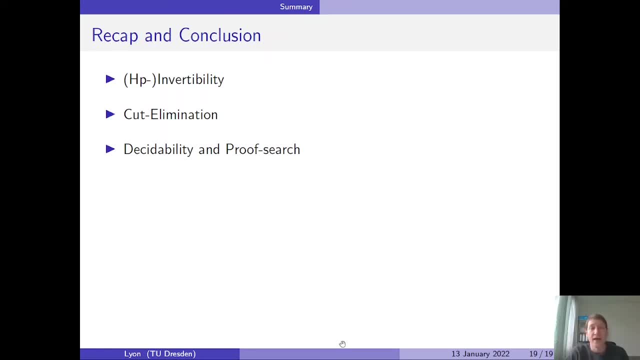 imply derivability of their premises, And this is a height-preserving version of invertibility, when deriving the conclusion with a derivation of a certain height implies that you can derive all the premises with derivations whose height is no bigger than the derivation of the conclusion.